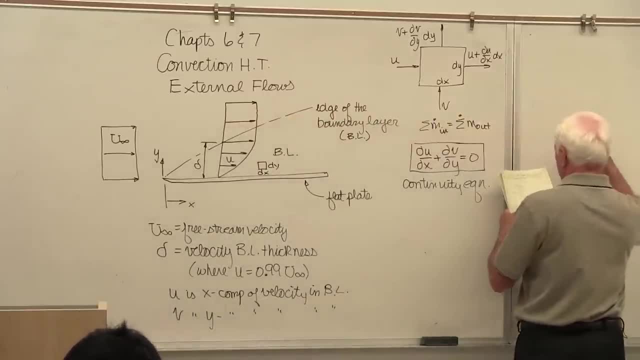 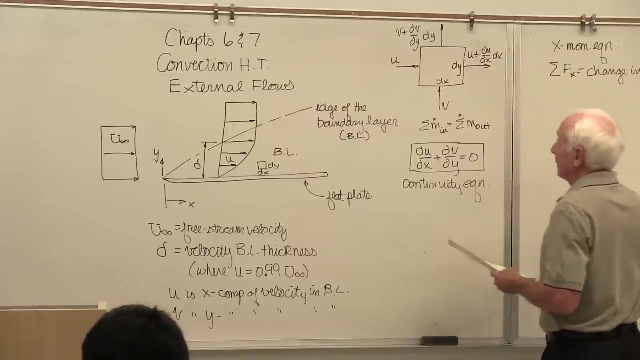 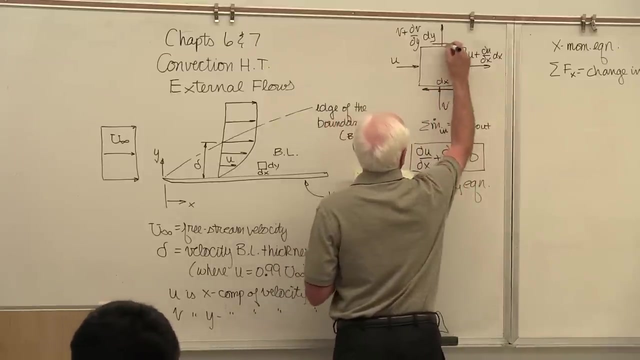 first equation. Second equation: momentum: X momentum equation: Summation of all the forces in the x direction equal the change in x momentum. The forces there are going to be the shear stress forces. So there's a force here and a force here. 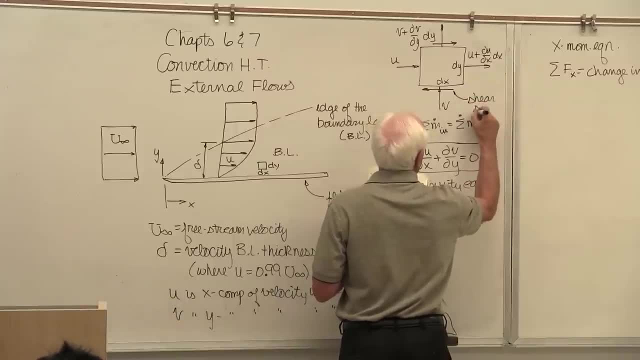 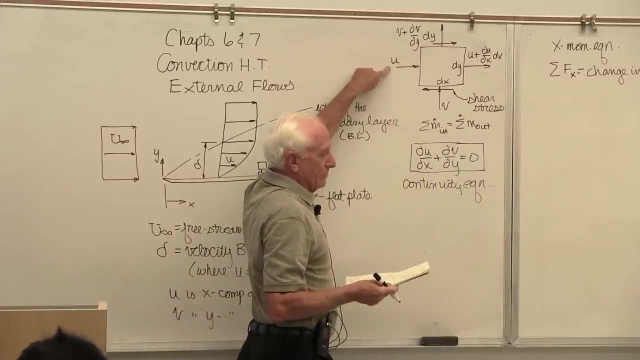 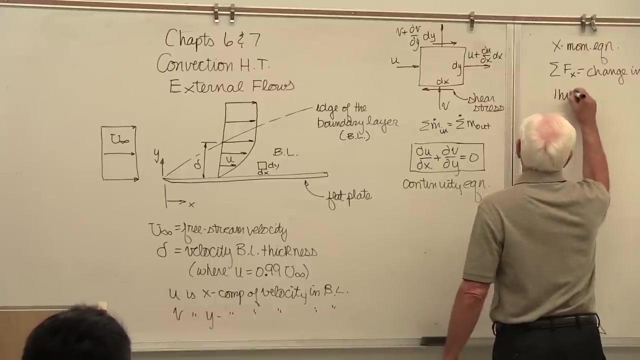 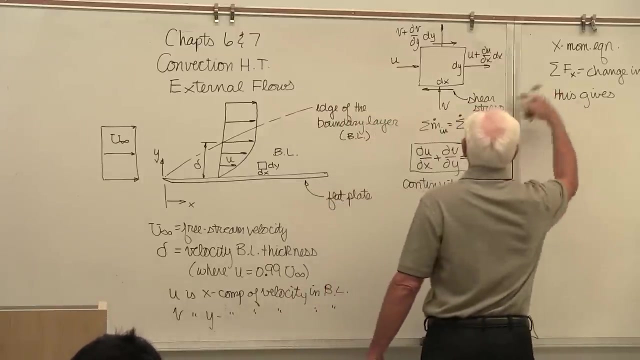 and this is shear stress. Okay, What's momentum? M dot times u, Mass flow rate times the velocity. Again, this was done probably in ME 312.. If you put that, in what forces are there The shear stress forces? 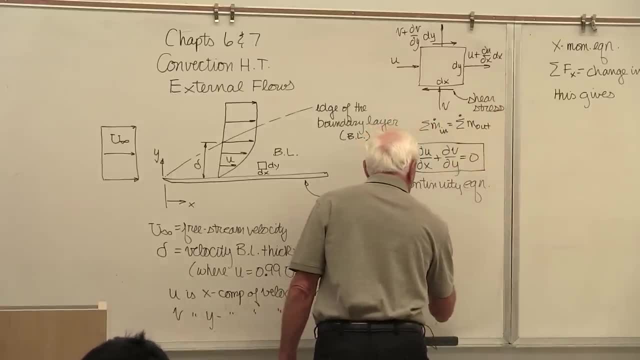 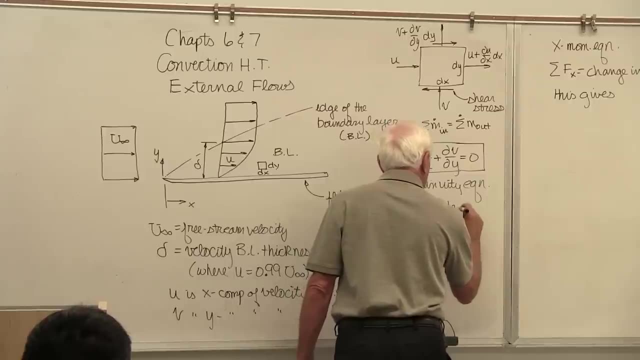 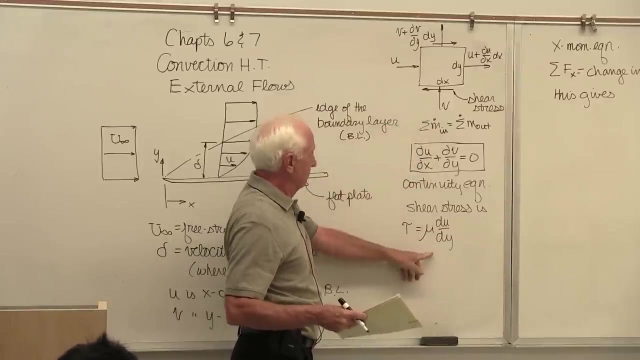 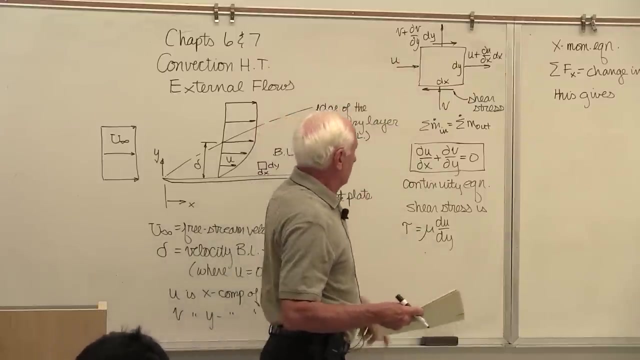 And the shear stress forces tau equal mu du dy. Okay, So you put that guy in there in the x direction And on the top in the x direction, different sign: Put it in there. You end up with this equation. 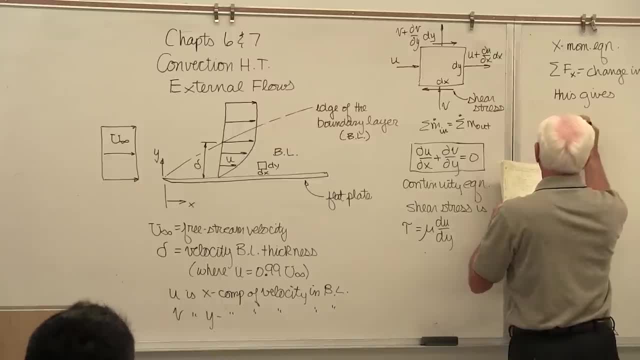 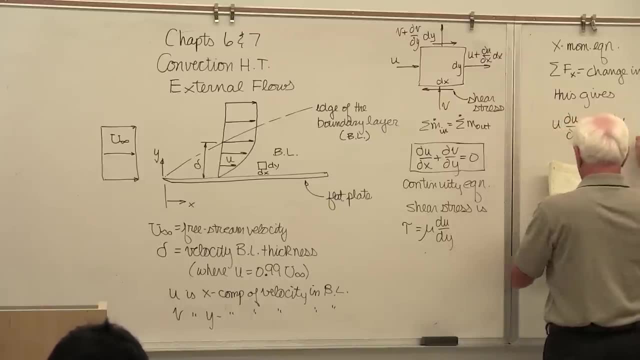 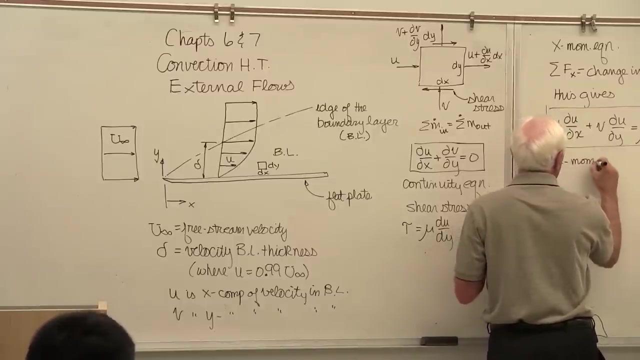 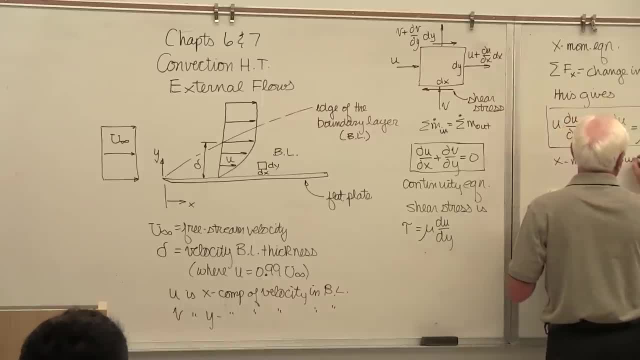 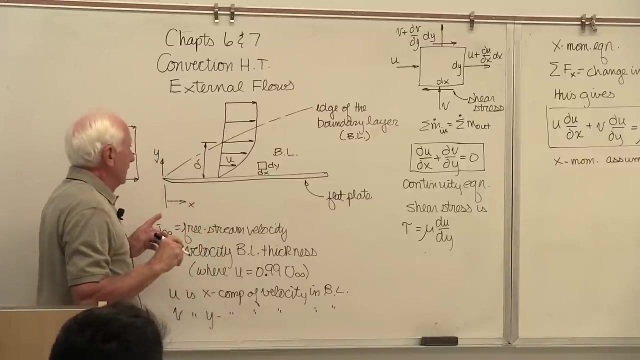 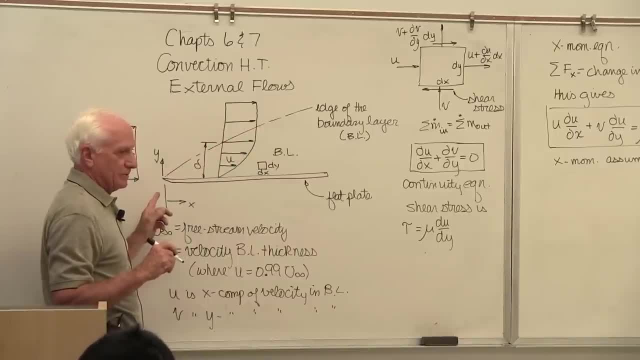 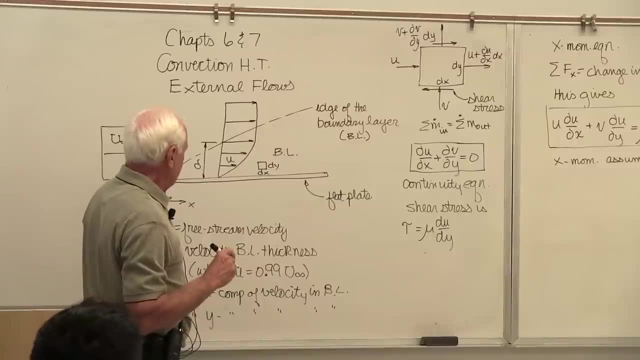 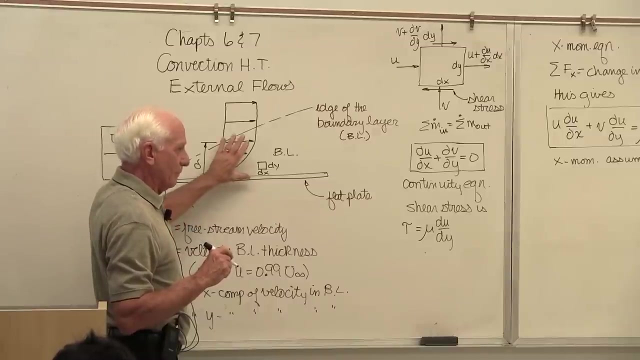 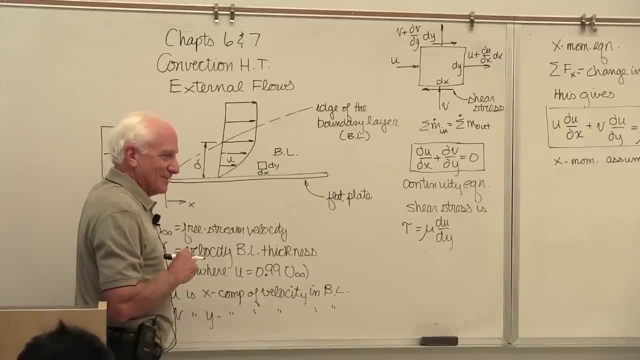 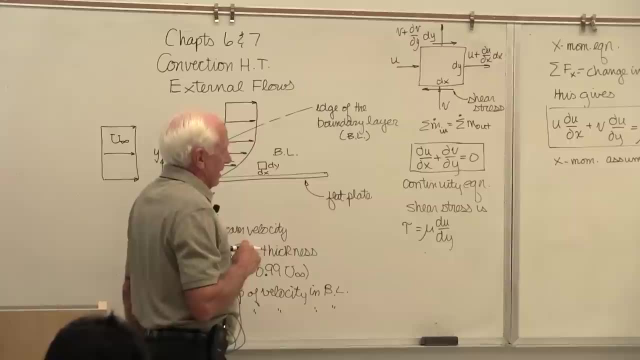 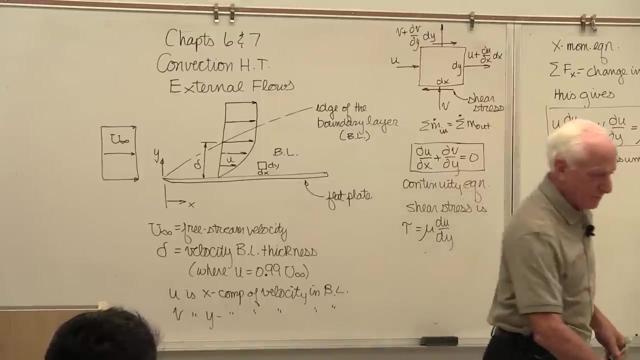 That's the boundary layer, It's where all the action occurs, That's where the shear stress is, That's what causes the drag, That very thin layer of fluid, The governing partial differential equations. Is P constant? Yeah, P is constant, Assume. 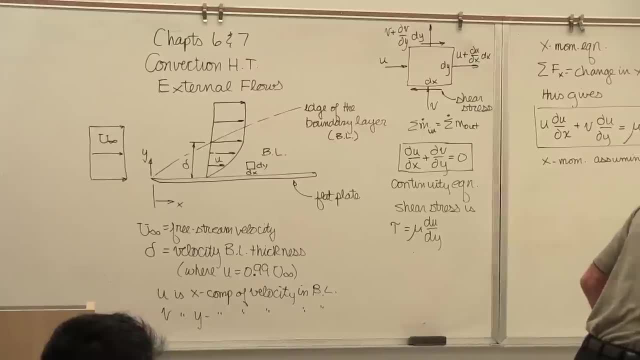 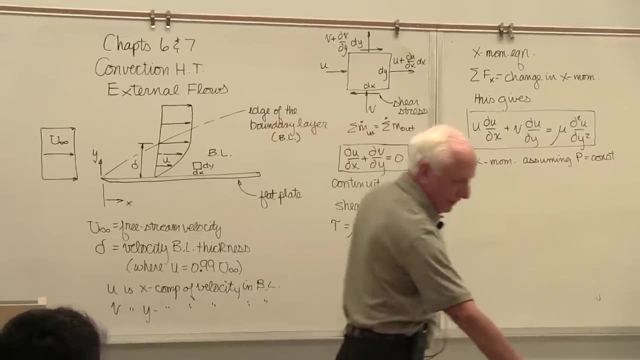 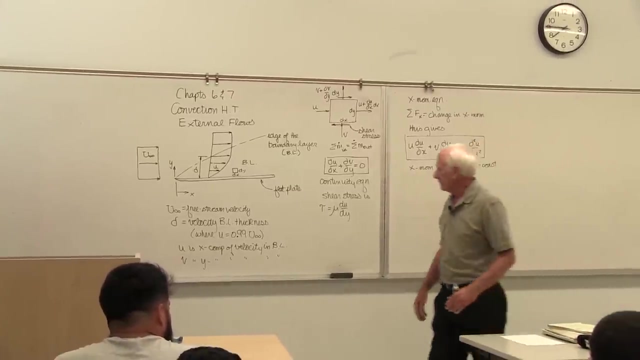 this is a flat plate here. This is X. that way, This is Y, that way, This is X0.. I put a floor fan here. I blow the air over that table. A boundary layer builds up from the leading edge and it gets bigger and bigger and bigger as X increases. Okay Is the pressure. 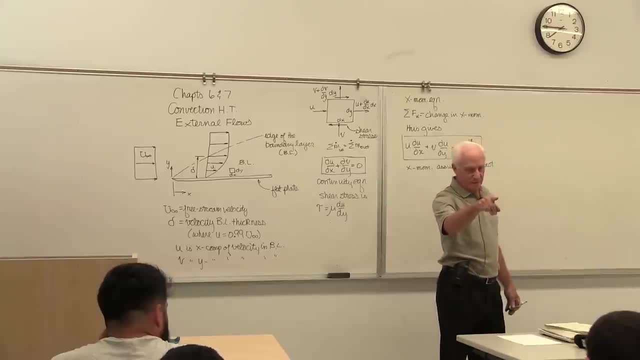 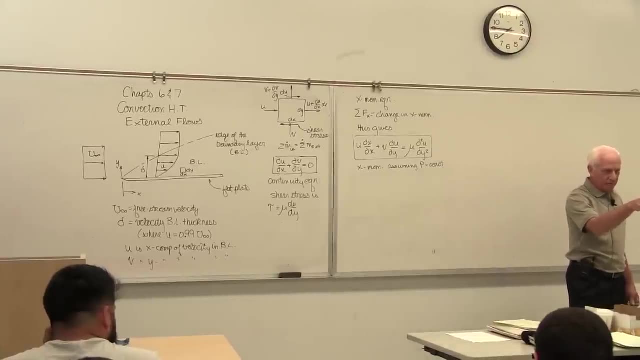 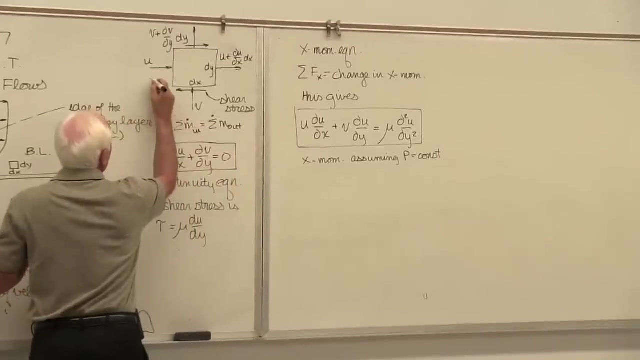 constant. The pressure at my fingertip 14.7 psia, In the middle of the plate pressure 14.7 psia And in the plate 14.7 psia. Yes, the pressure is constant. Okay, If it's not constant, there's. 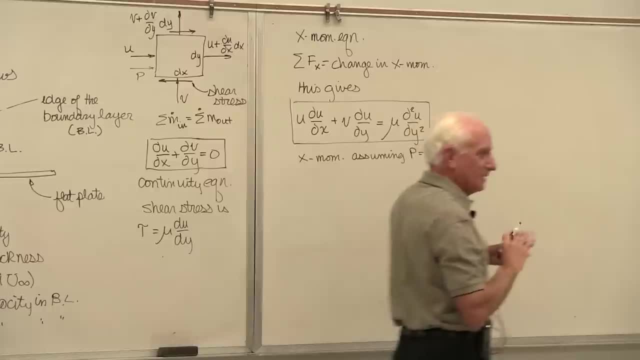 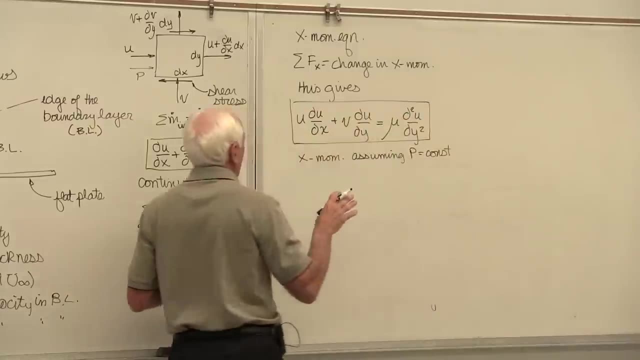 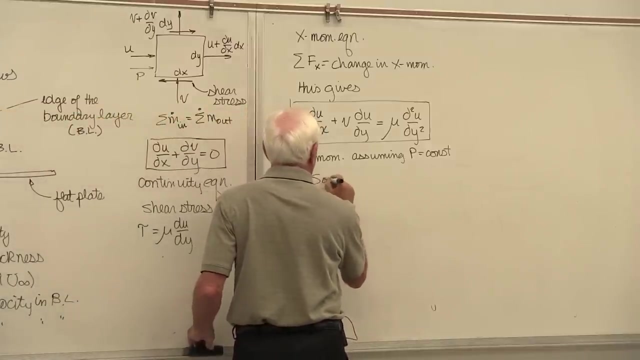 going to be a pressure force in the X direction. No, it's constant, It disappears, It's gone. Okay, So that's it, These two equations, the unknowns. well, look at them: V and U. We want to solve for U. 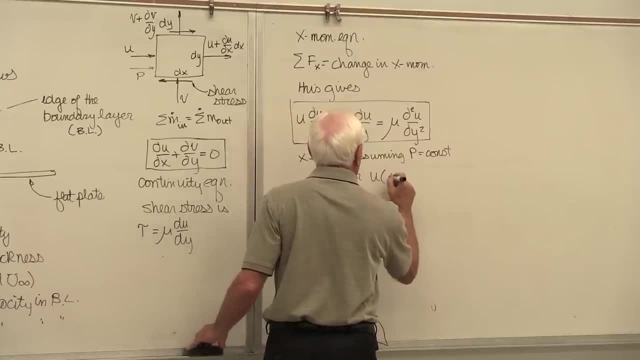 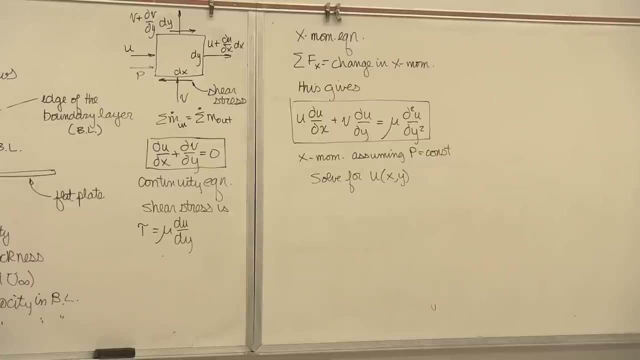 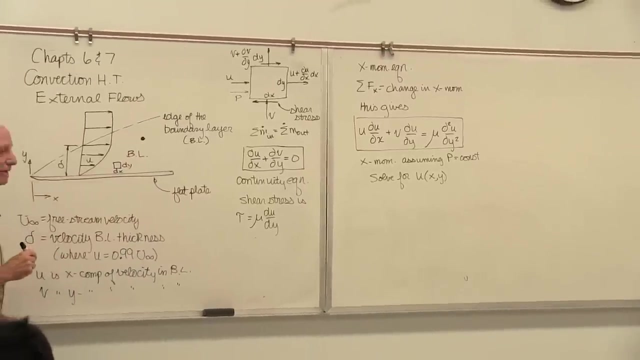 U as a function of X and Y. Where is it in the picture? Right here, Right here. Put any point you want in the boundary layer, That big fat black dot. Tell me the velocity there. Okay, That's what the solution gives you. I give you an X and a Y and hopefully you. 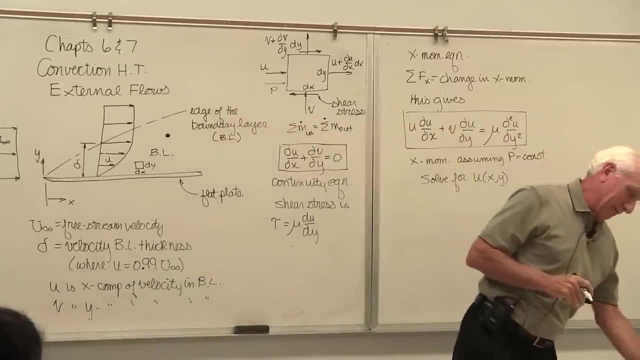 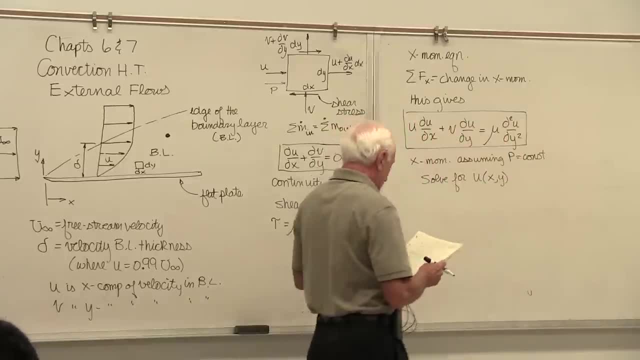 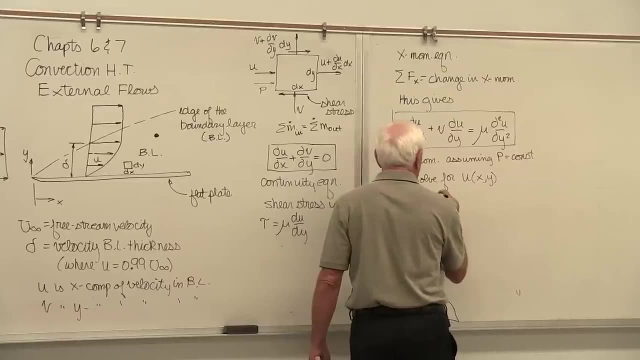 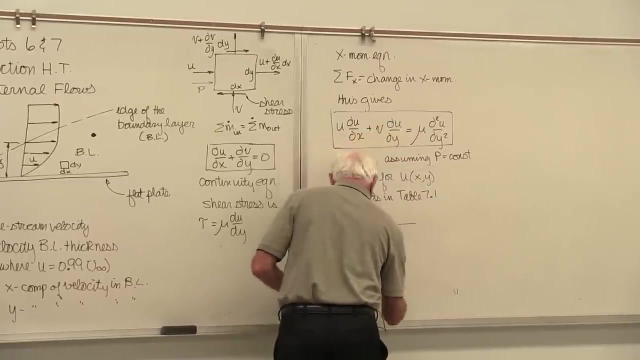 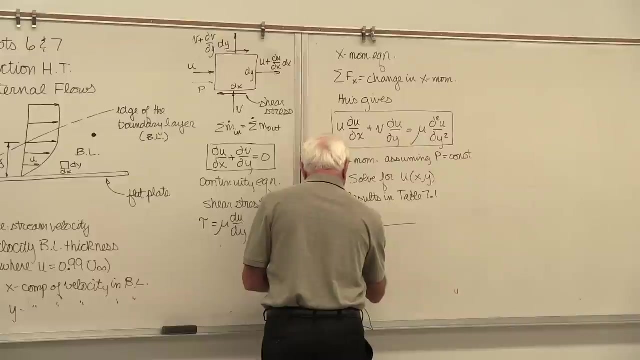 Normally you don't go through all the gory details, But anyway, the results are in Table 7-1. in our book, Table 7-1 looks like this: The first column is this: The second column is: little u over u infinity. 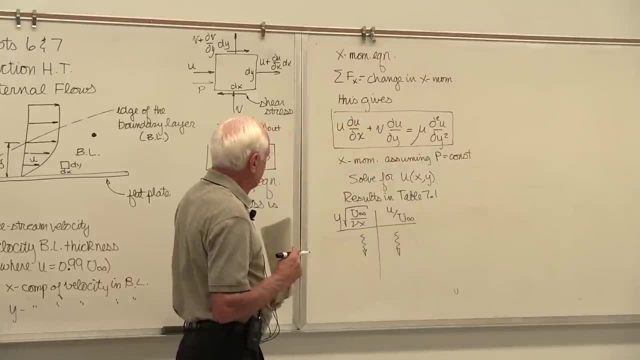 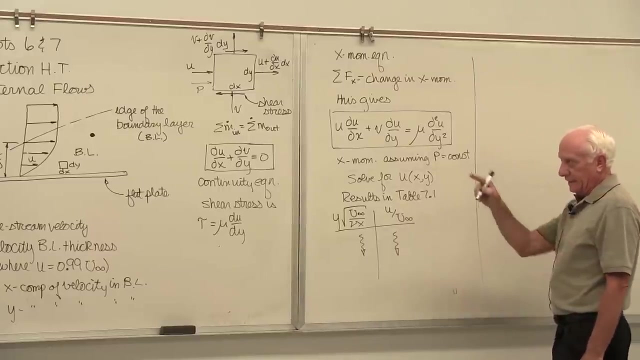 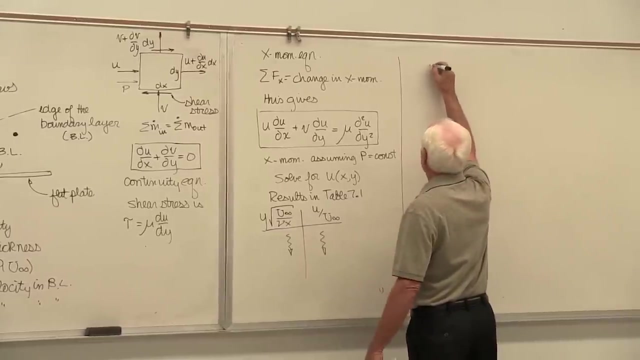 Okay, Okay, Okay Okay. There's u, there's x, there's y. So what we do now is we say, okay, I want to find out what delta is as a function of x in that picture, So let's solve this for delta. 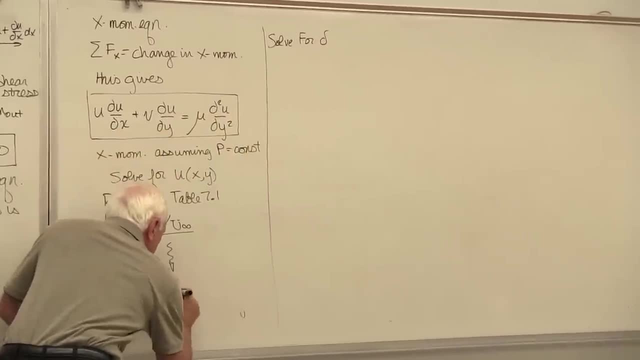 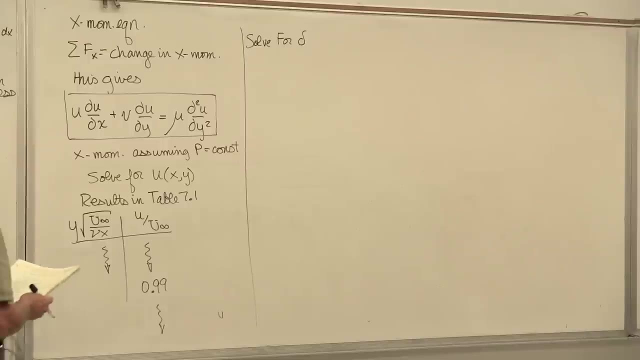 Now, where's delta? Delta is where u over u infinity is. U over u infinity is 0.99.. So go to the table 0.99,- this is what you would do, And then over here you'd find a value of 5.. 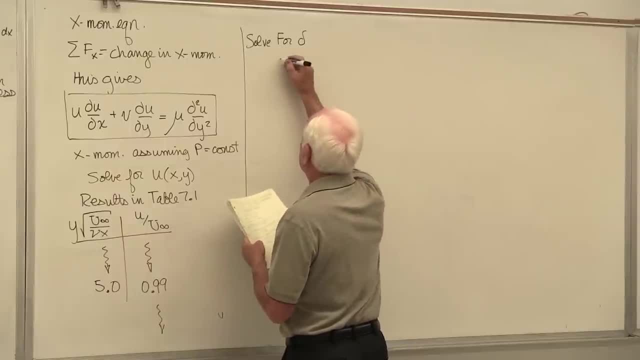 So what we have here, then, at u over u infinity, 0.99,. then this column: And what is y? y at that 0.99.. y is delta, Delta, square root, u infinity over nu x equal 5.. 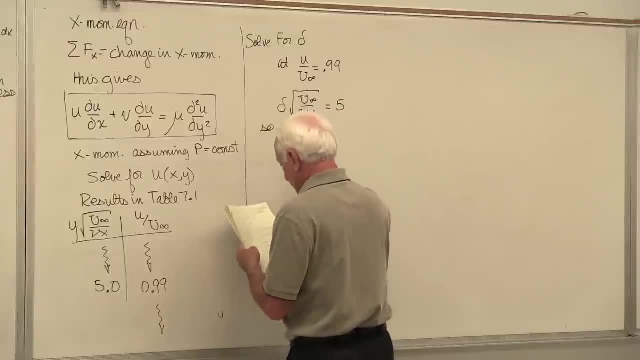 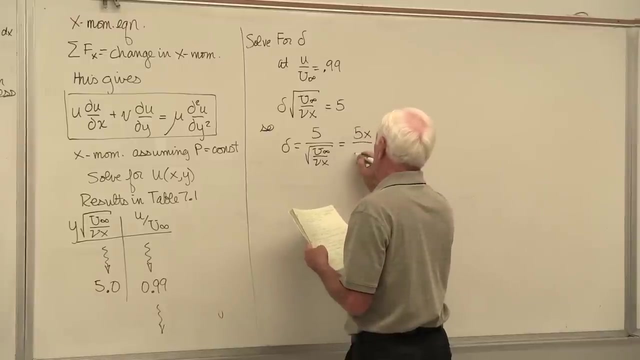 Solve that guy for delta. So delta is equal to 5 over the square root u infinity, nu x, which turns out to be 5x over the square root of the Reynolds number. So delta is just a minus. And so delta is equal to 1 over the square root u infinity. 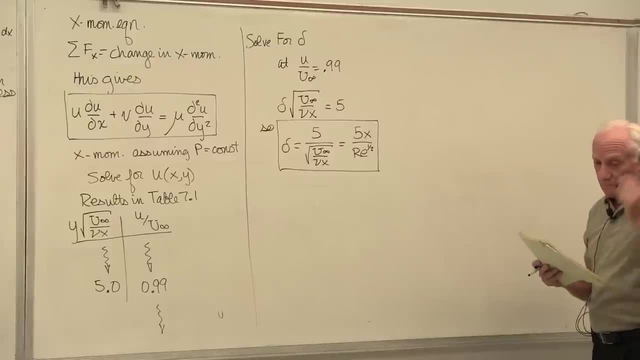 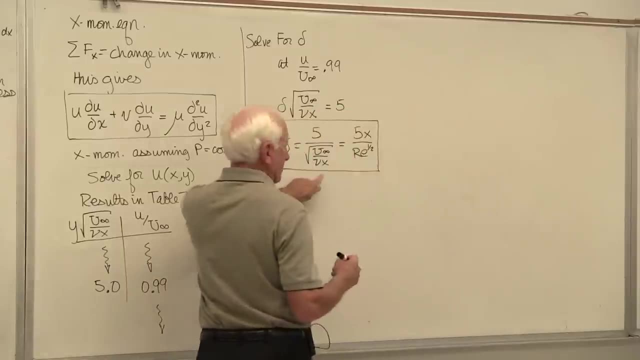 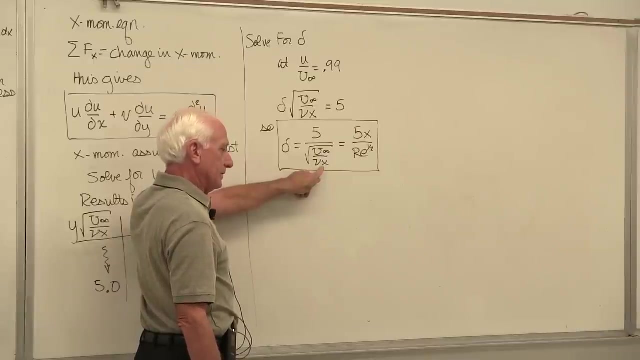 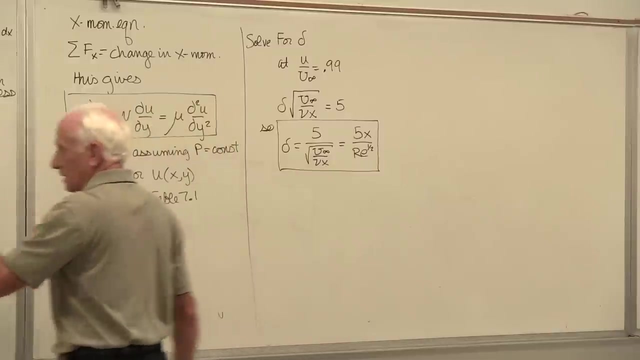 nu x, d, x, Delta is equal to negative. So here's the equation right here. All right At: x equals 0, delta equals 0.. As x gets bigger, delta gets bigger, bigger, How? As a square root of x here Bends over like this, Square root of x like this: 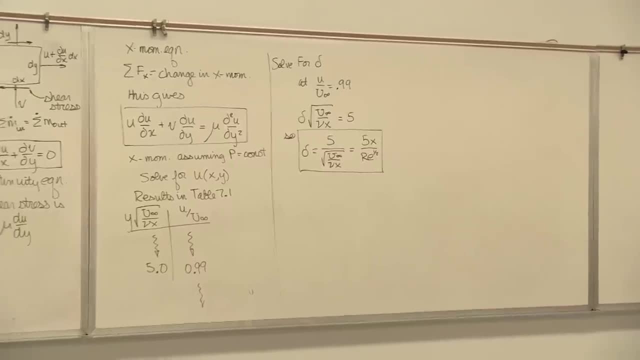 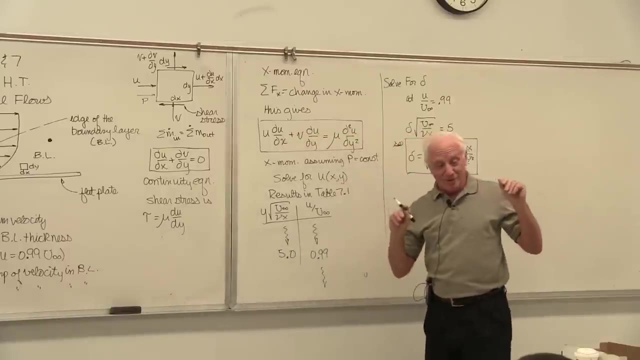 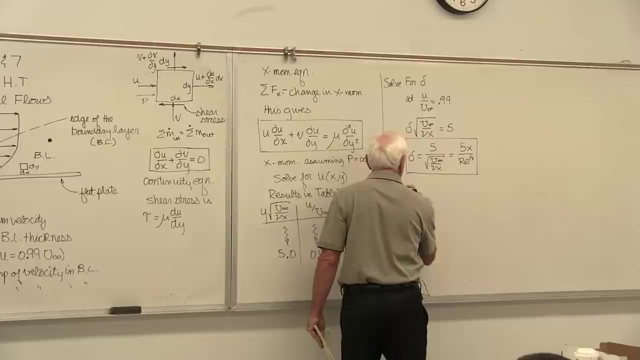 It's not linear, It bends over as a square root function. Okay, so that's how we find- quote- the edge of the boundary layer. Now, in ME 312, we're interested in finding shear stress and drag. So shear stress, tau equal, mu, du dy, And we're going to do that at the 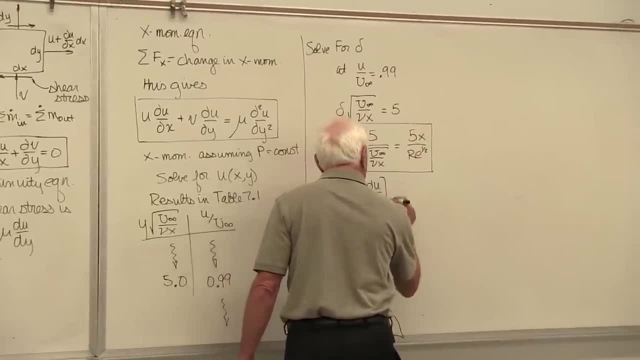 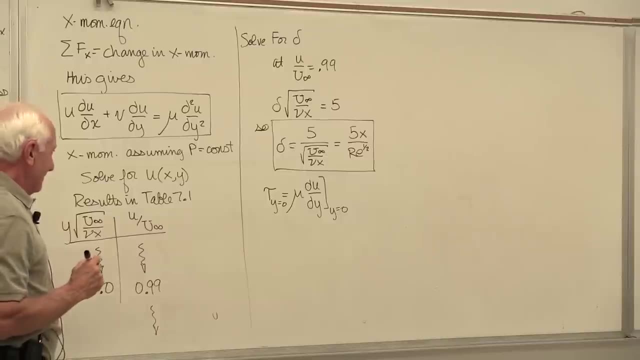 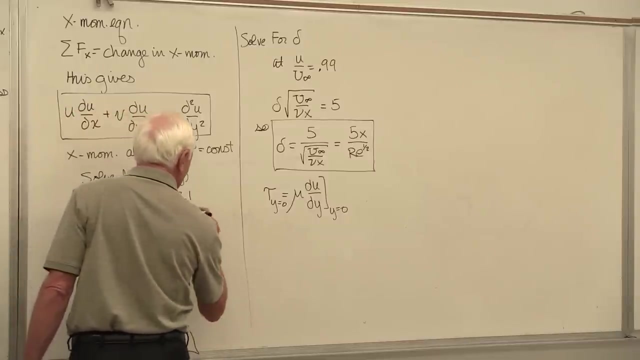 surface Tau at y equals zero. Evaluate du dy at y equals zero. There's another column in here which gives you: if you work it out, it'll give you like du dy. Okay, If you go in there and do that, you end up with this. 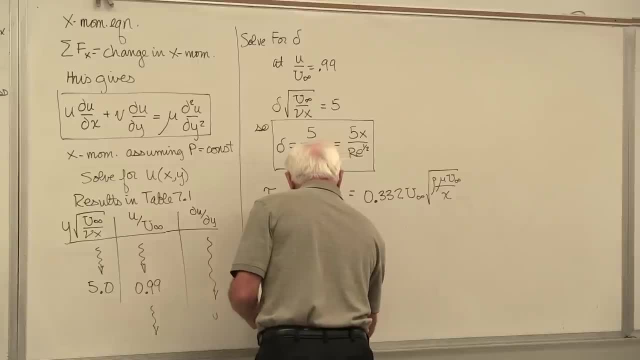 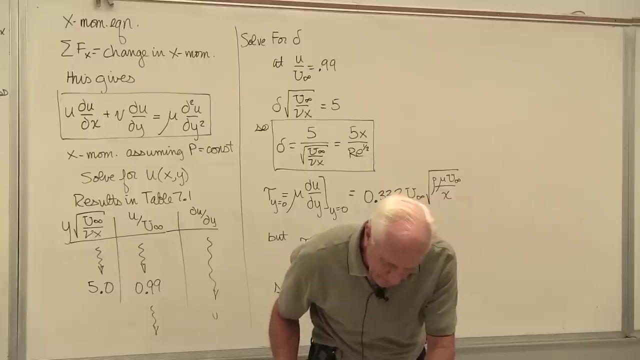 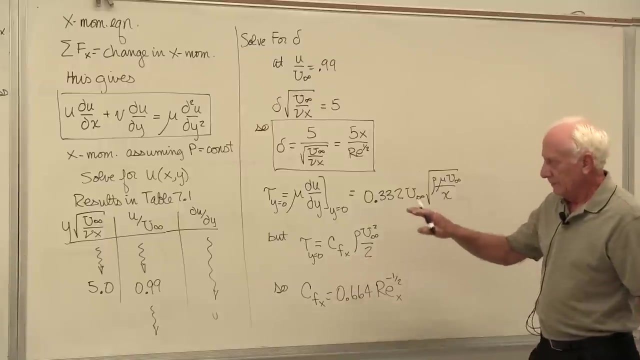 Okay, so we're going to do that, Okay, Okay, Okay, Okay, Okay, Okay. And let's see here: Yeah, Mathematically, that's how you get the shear stress at the surface of the plate. There it is. We engineers use this equation. This equation says the: 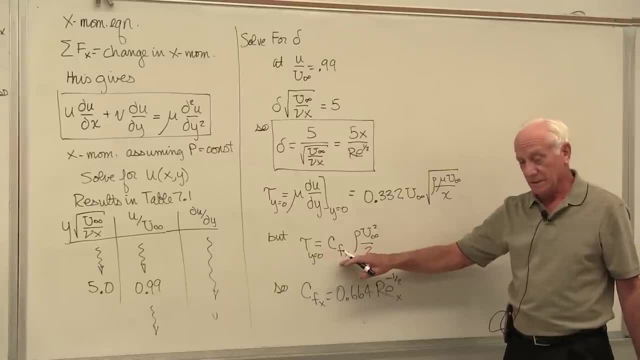 shear stress at the wall is a constant. that's the constant times. rho U infinity squared over 2 kinetic energy, a constant times the approaching kinetic energy. That constant is C sub fx. the f stands for friction, the x stands for location, the c stands for coefficient. 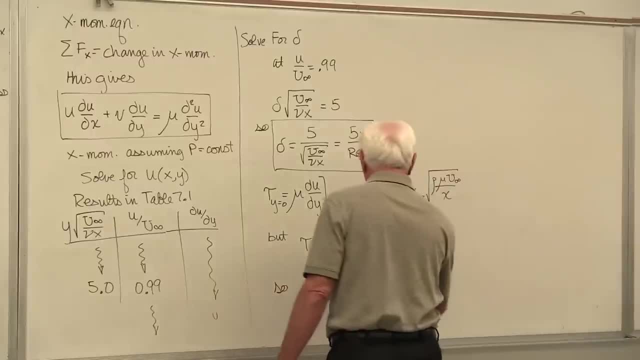 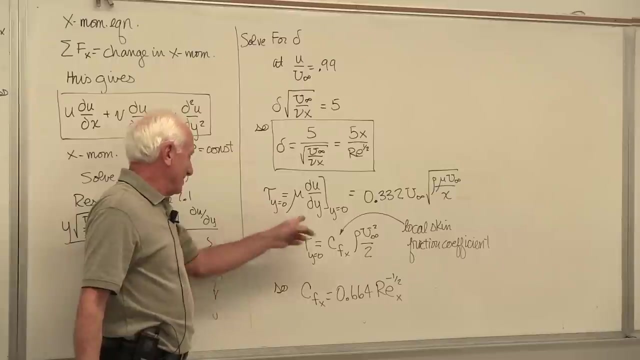 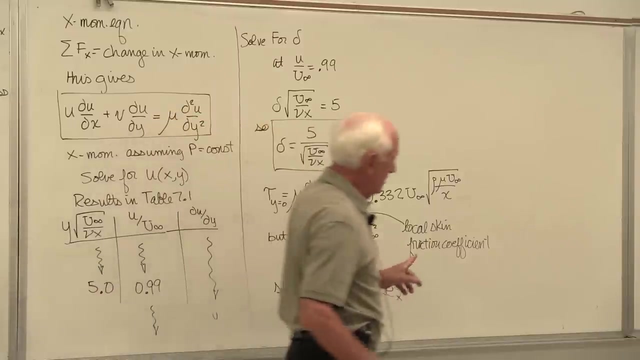 So that is titled the friction coefficient. So C fx is titled the local. really it's called the skin friction coefficient. The real way you get the shear stress is here. This is the equation we engineers invented. Is that something that came from the basic principles of the governing partial differential? 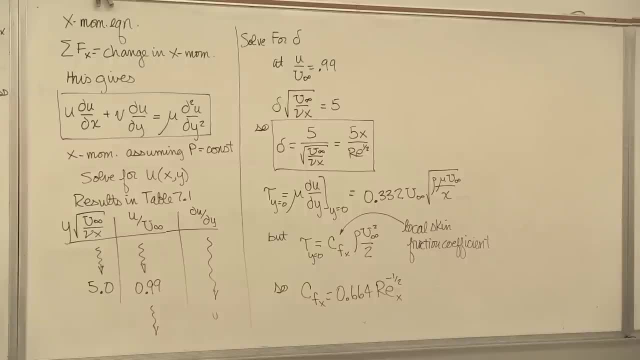 No, Okay, The differential equations, my gosh. no, It's the Darcy-Weissbach equation. Who invented it? Here we are, we engineers, we invented it. Why did we invent it? Because it's simple. 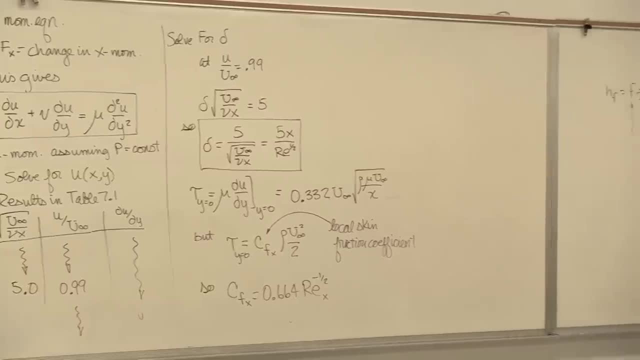 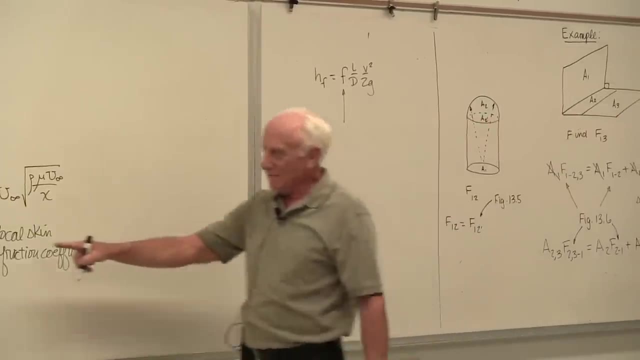 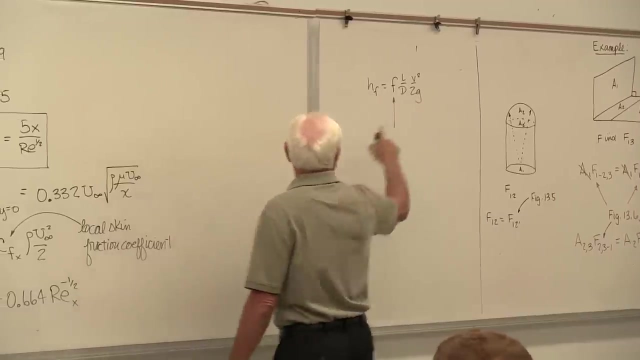 There is something called a friction factor that takes into account all the messy stuff And when you want to find the head loss due to friction, that's what you use Here. we invent this because it's very simple, very simple: a constant similar to that Look. 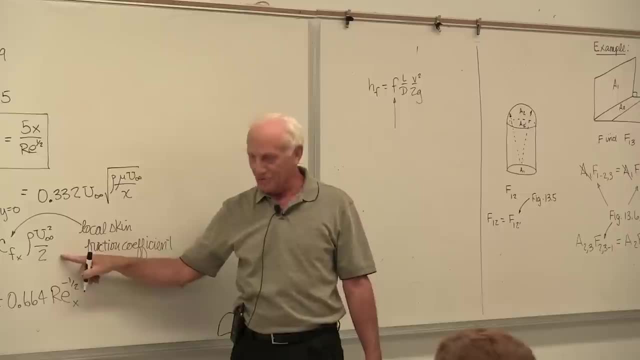 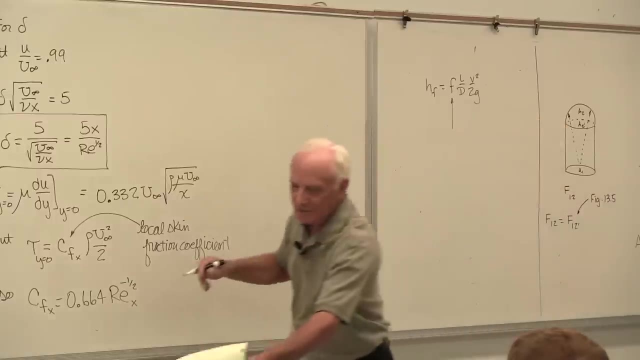 at the v2g. look at the v2g. it's the same thing almost, except that's the constant. now, What's that guy called The local skin friction coefficient? So we take these two equations, we equate them. see that right. see the two right there. 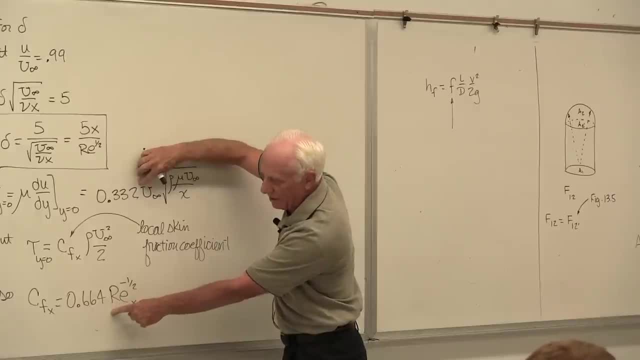 See the 332?. There it is 6.64,. okay, And so this is how, in ME 312, we found the skin friction on the surface over there. If you want to integrate that, then multiply it by an area. you're going to get the drag. 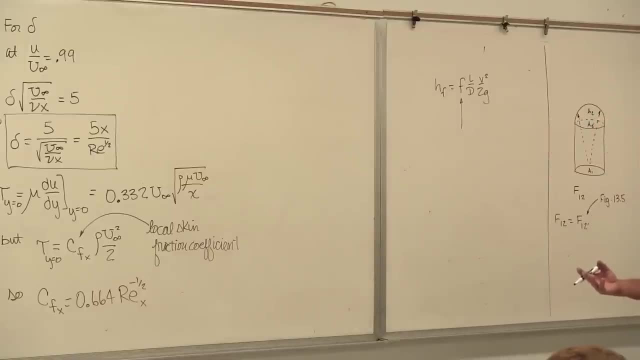 force on the plate. Okay, ME 312, one more time: Okay. so that's where we kind of ended up. start off with fluid mechanics. Now we have to shift gears. We're no longer looking at the velocity boundary layer. 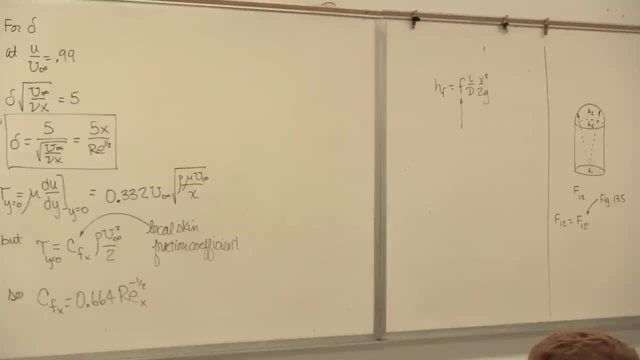 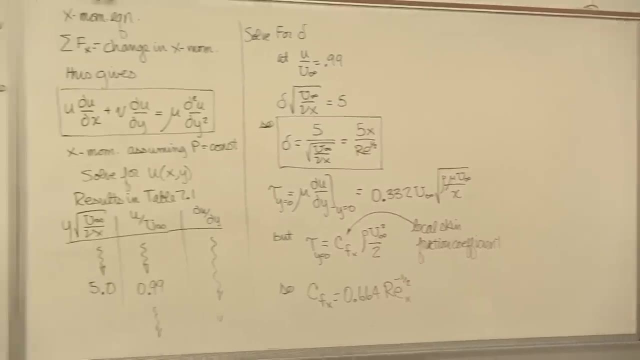 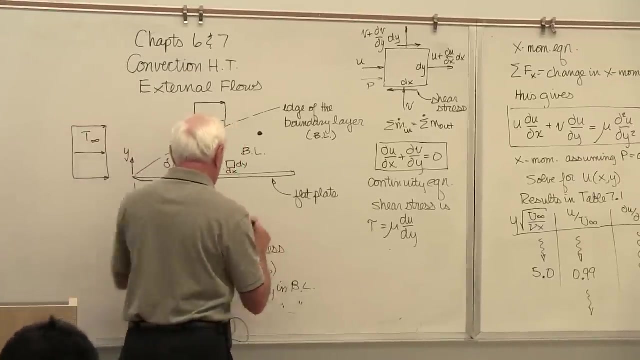 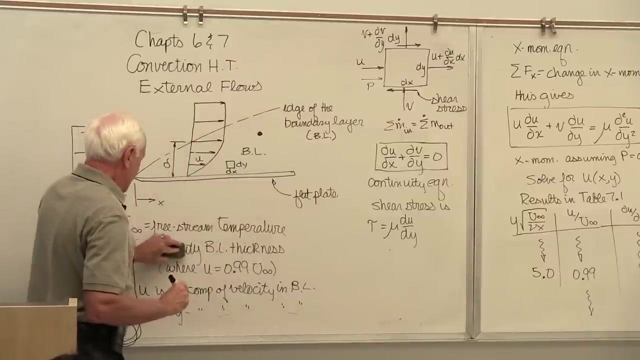 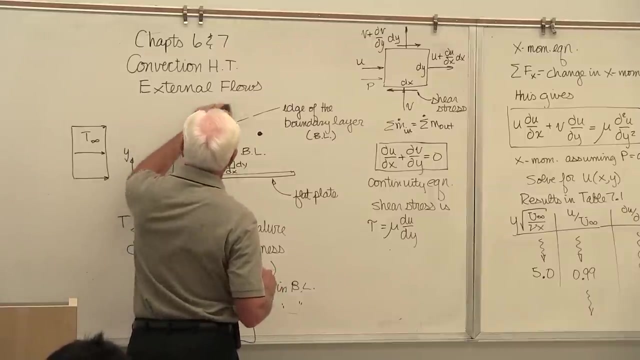 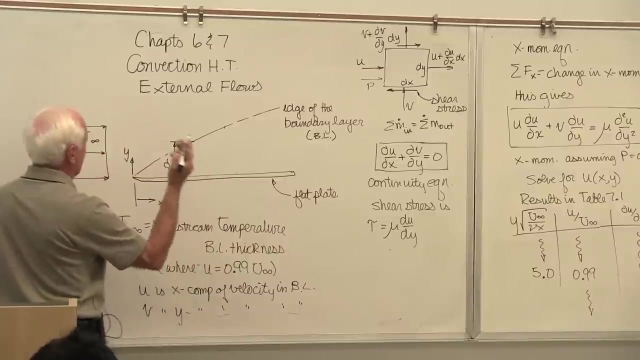 This is heat transfer, ME 415.. We're interested in temperature, So now we change things. This becomes the approaching free stream temperature, T infinity, the free stream temperature. Okay, Here is what happens. Okay, I'm going to, just for the sake of argument, I'm going to say TS is greater than T infinity. 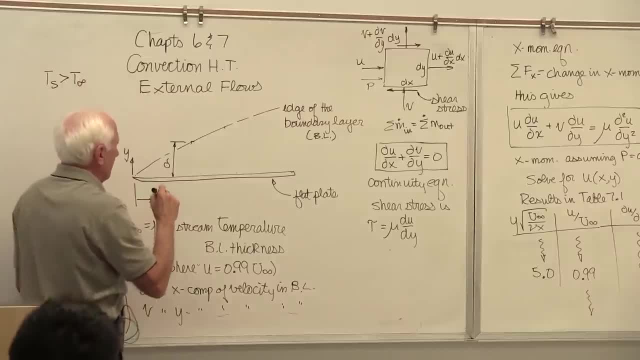 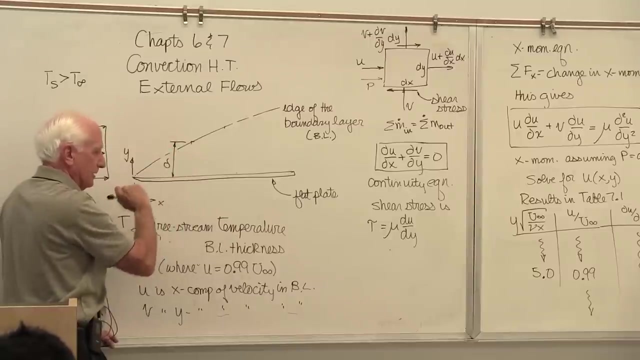 The plate's hot, the fluid's cold. The plate temperature never changes with X, It's a constant TS, T. infinity is outside, far away from the plate. The temperature changes from the surface temperature of the plate to the free stream in the Y direction. 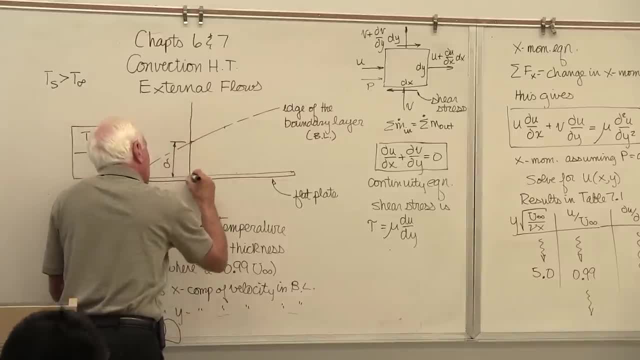 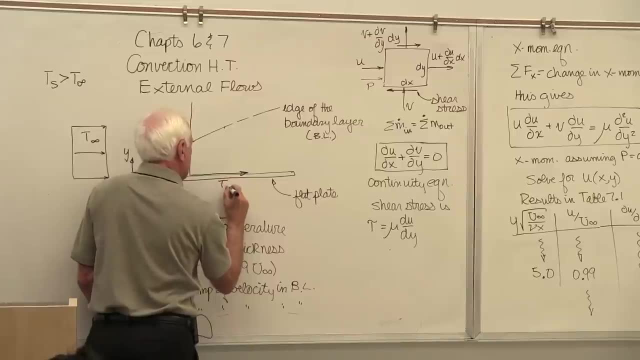 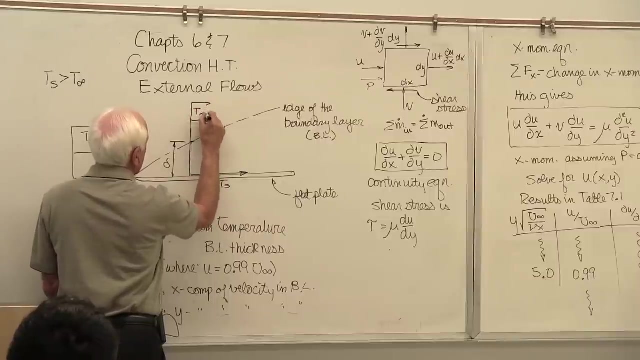 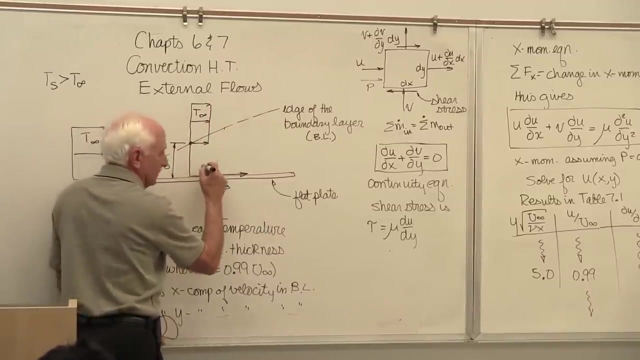 Okay, Let's plot how that might look. at any X, at any X Surface is hot. Okay, So this arrow represents the surface temperature, TS. The free stream is colder. All right, We'll represent that as T infinity. Now you connect them- not linearly, of course, like this: 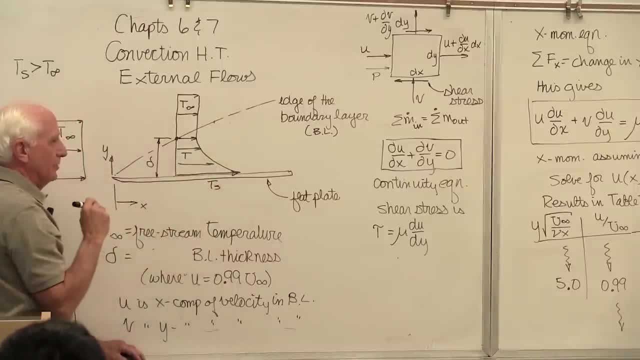 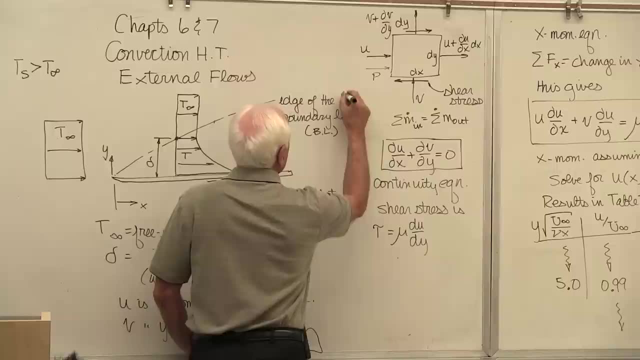 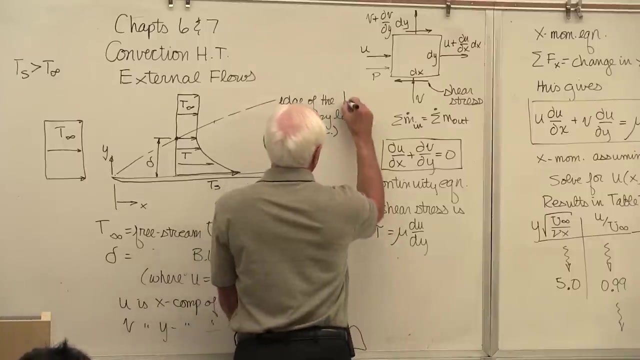 Okay, And this is the temperature in the thermal boundary layer. T is the temperature in the thermal boundary layer. This line now represents the edge of the thermal. we'll make it temperature. Either call it a thermal or temperature boundary layer. We'll call it temperature boundary layer. 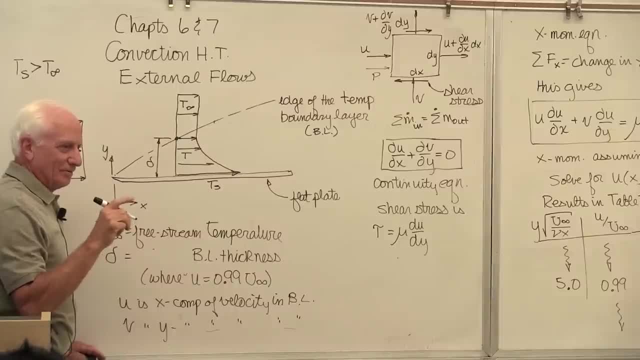 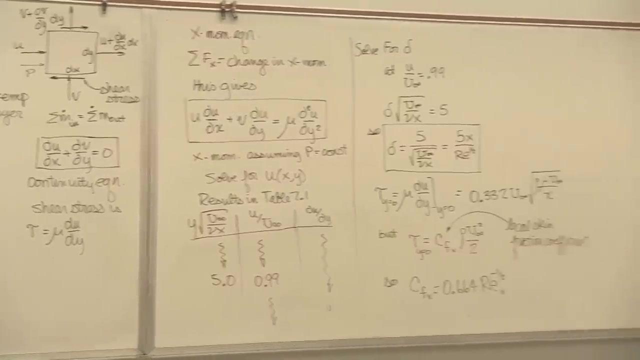 So now the boundary layer thickness is still defined by 99%. Okay, Okay, Okay, But now we call it delta T. The T stands for temperature, So delta T is the temperature boundary layer thickness. now, If I'll just show you the other picture, 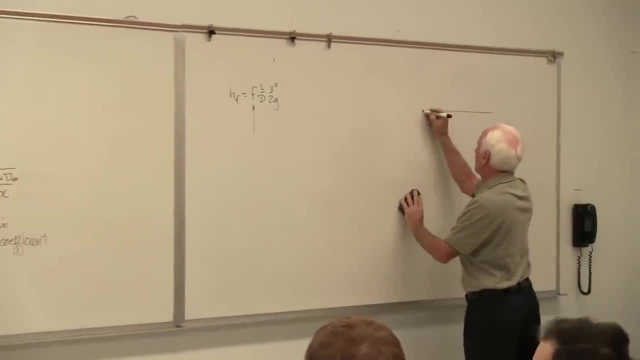 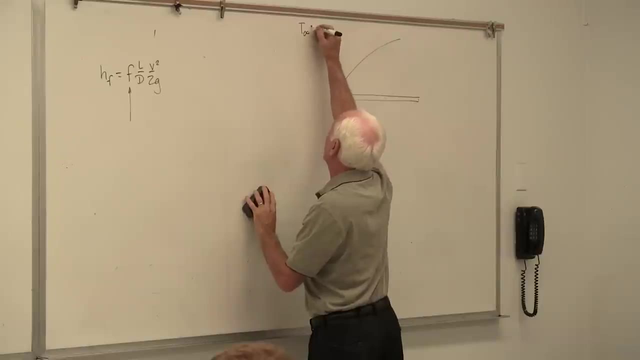 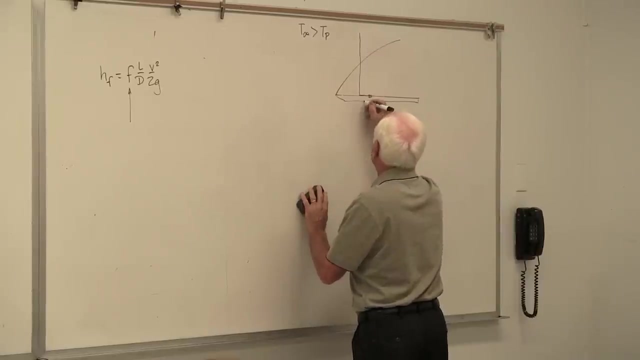 If we have the opposite case occurring in the plate- Okay, Where, in this case, T infinity is hot and the plate is cooler, then here's how it looks. Here's the plate. surface temperature- TS stands for surface temperature. Here is T infinity. 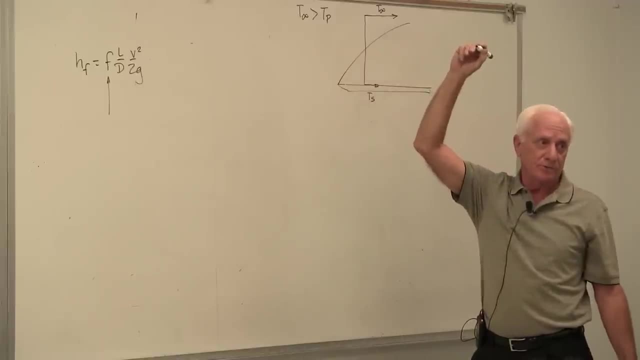 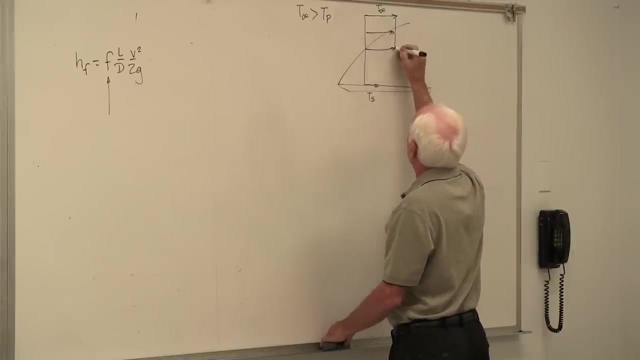 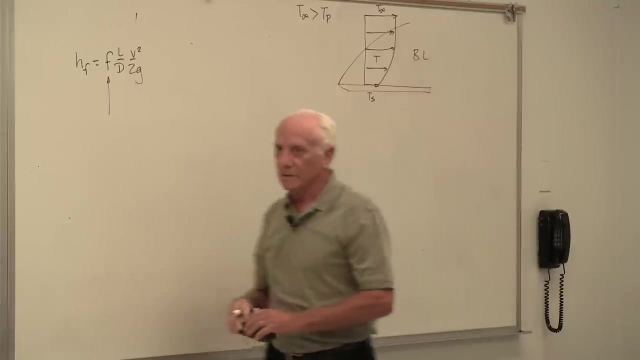 This might be in a gas turbine engine. hot gas is Cool. surface Comes down here. down like that There's the temperature in the boundary layer T. They both are analyzed the same way. You do it by dimensionless temperature differences, But the equations are the same. 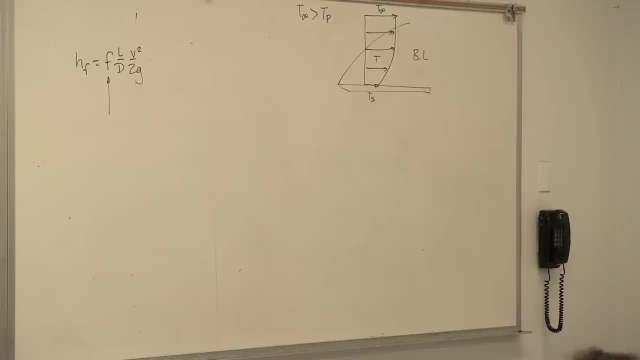 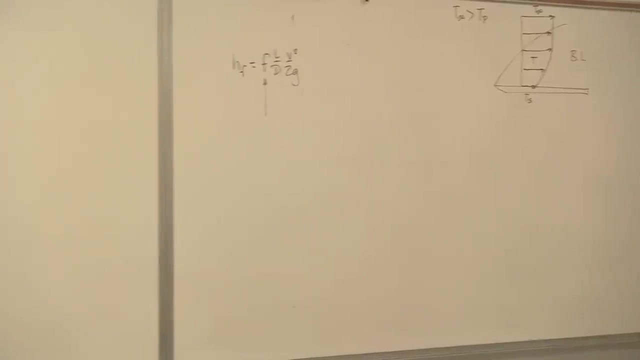 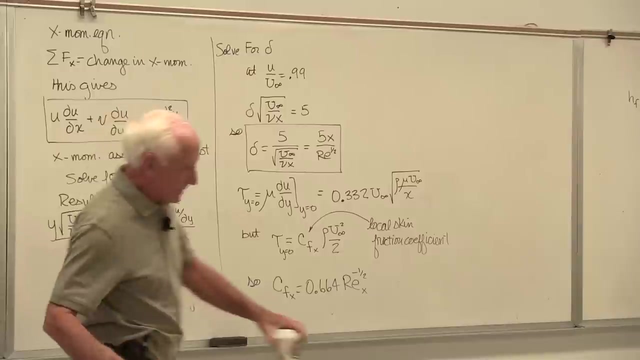 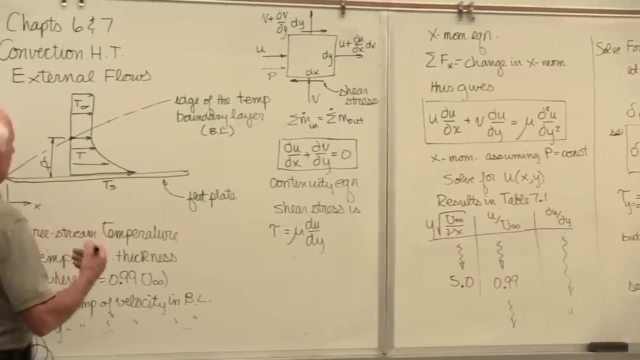 no matter which case you've got, So you can look at either case and then the other case is identical in the equations you're going to get. Okay, so now that's our picture. We still have U and V. of course, We still have our approaching. 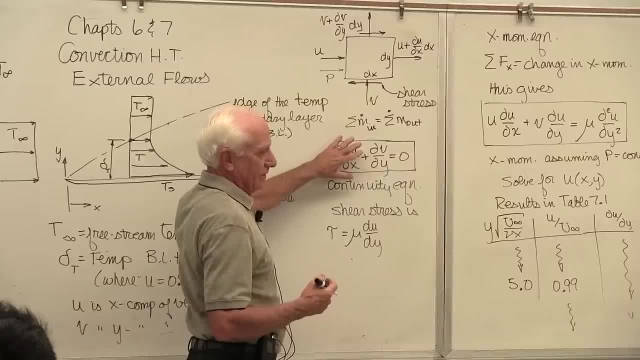 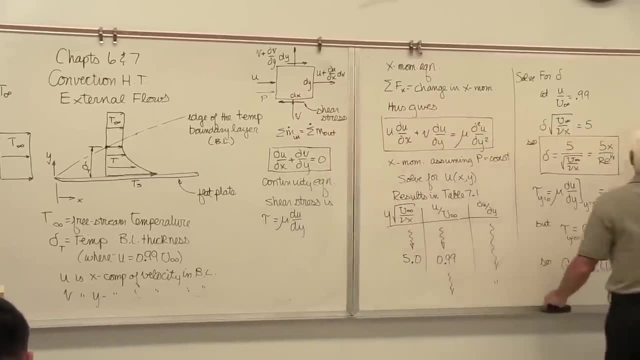 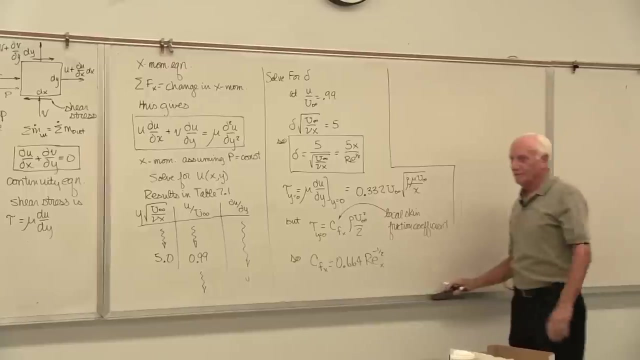 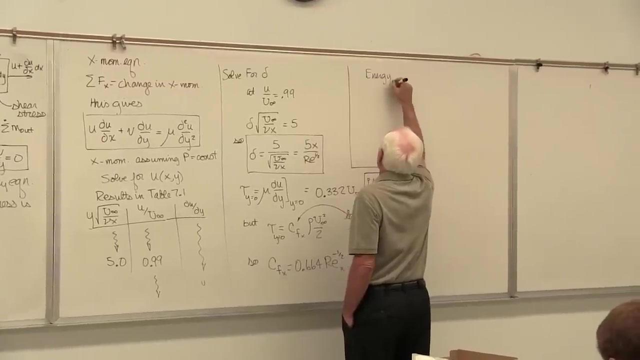 stream. We still have continuity, That's not going to change. We still have X momentum, That's not going to change. But Okay, Now we've got something different. You know what it is? It's energy, Okay, So energy balance. 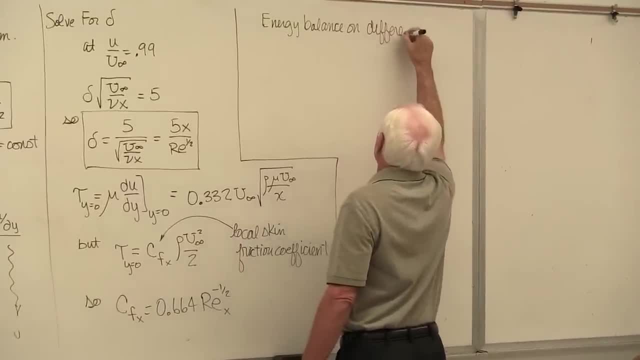 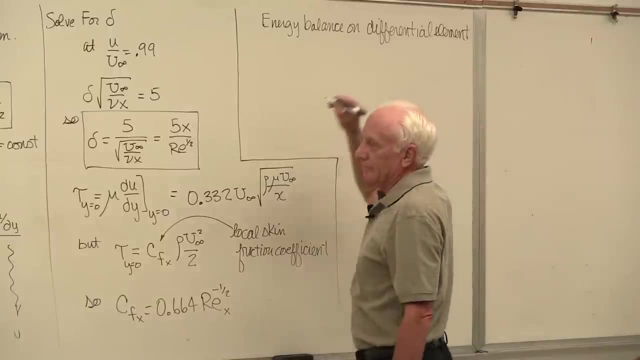 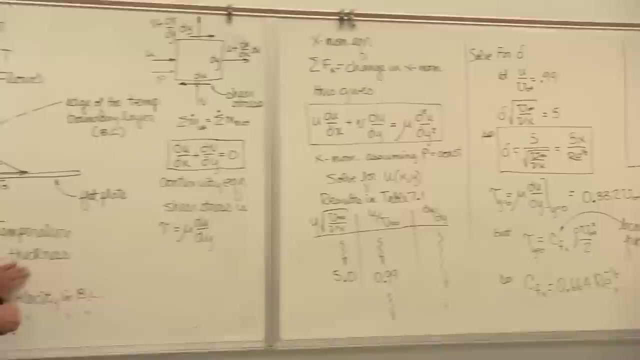 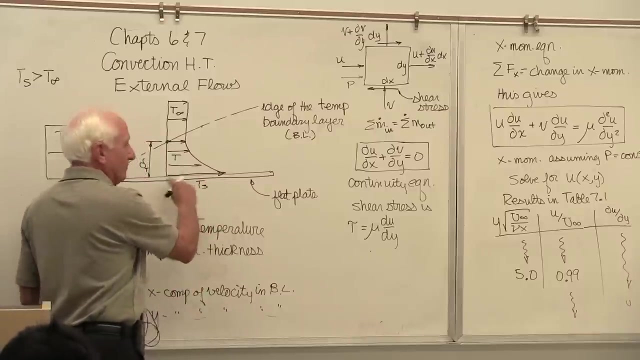 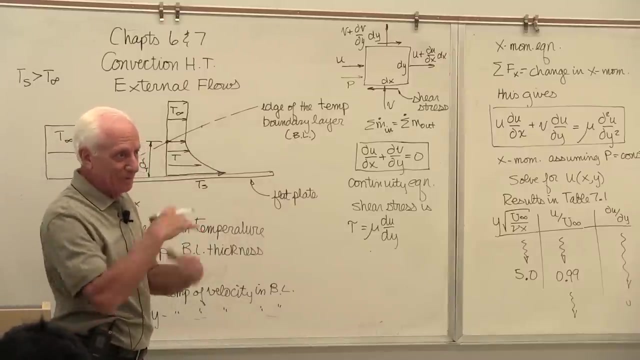 on differential element We take: Yeah, It's going to be a temperature difference. Okay, T minus TS divided by T, infinity minus TS is 0.99.. Okay, So it's a temperature difference: 0.99.. This point here is where the temperature 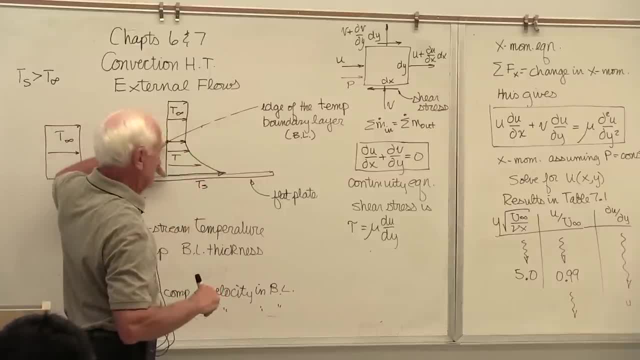 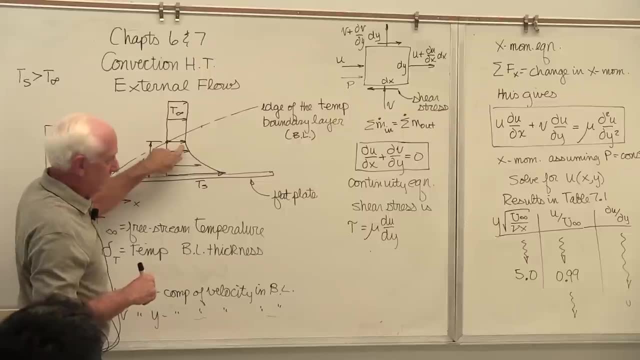 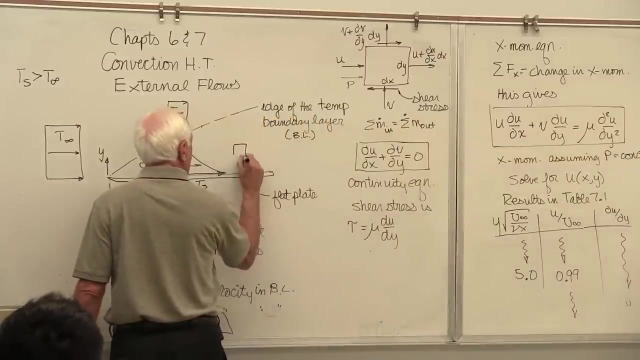 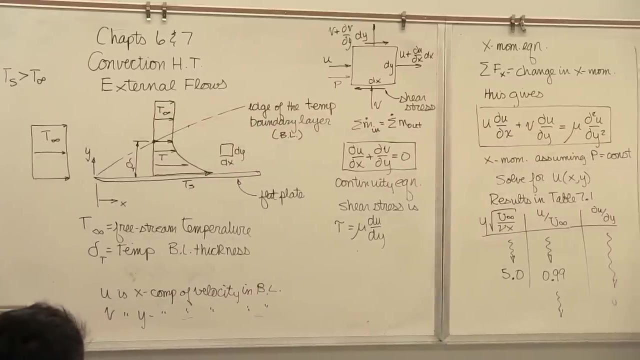 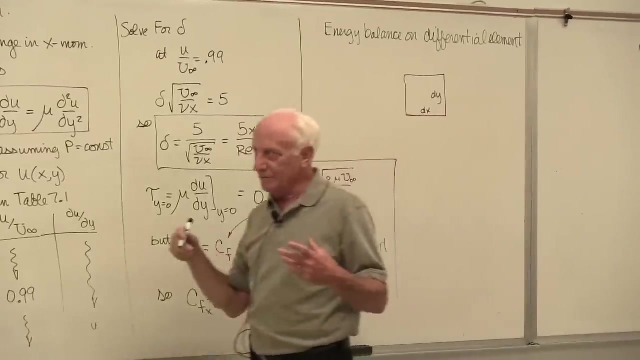 0.99 of this total difference. If this difference is 100 degrees, you're within 1 degree, right there? Well, take out our small differential element DXDY over here. DXDY, Okay, All right, All right, See, we do it the same for all three things: For conservation of mass, for momentum, for. 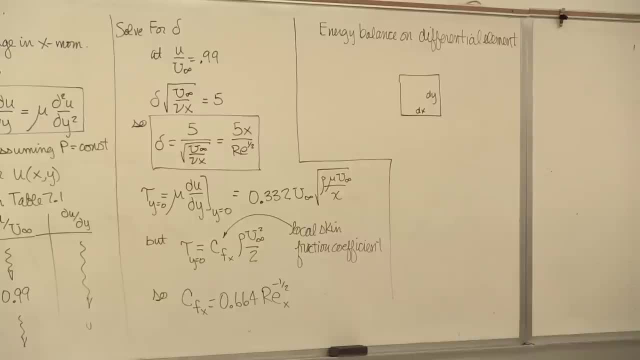 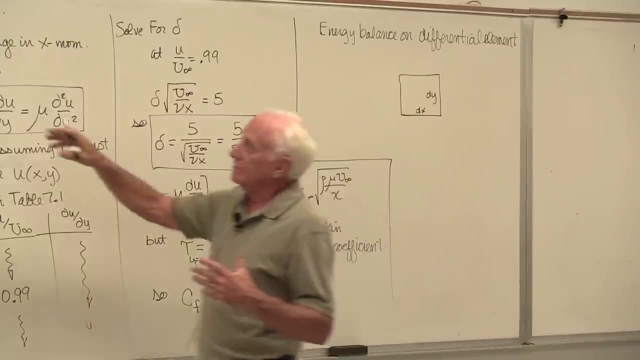 energy. the way we start to derive the governing partial differential equation is to look at a small differential element and look at whatever you're interested in crossing here: The mass coming in, the mass going out, the change in momentum, the forces on the differential. 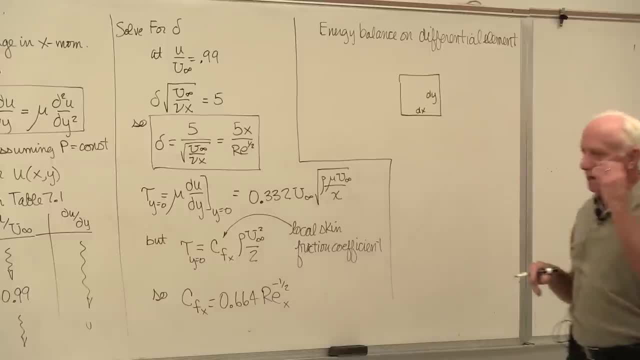 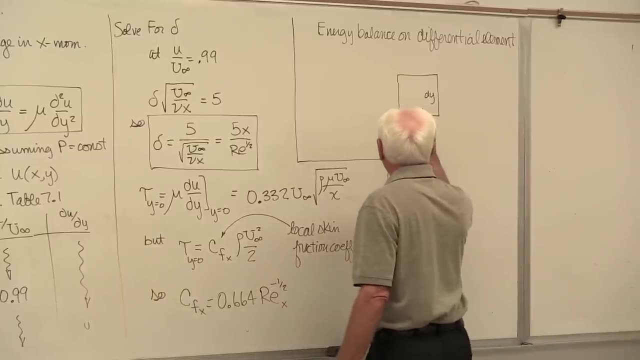 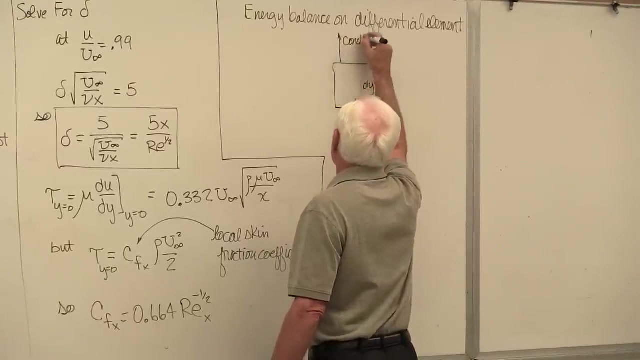 element Over here. energy coming in and going out. All right, let's take conduction here, Conduction out. Why is there conduction? Well, look at the picture. Does the temperature vary in the y direction? Yeah, it does, It varies in the y direction. 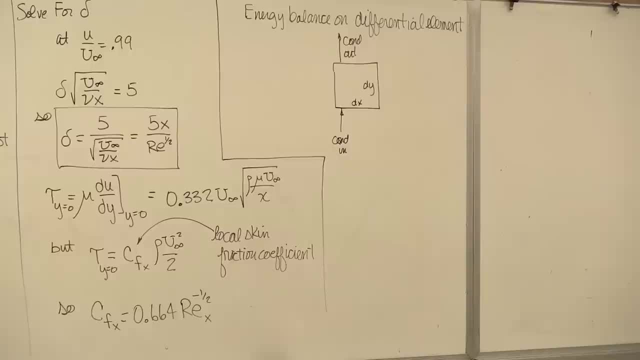 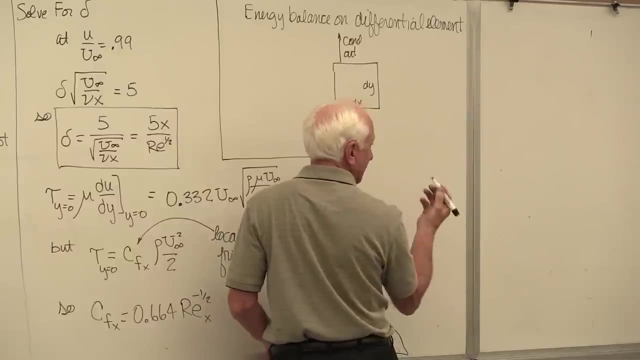 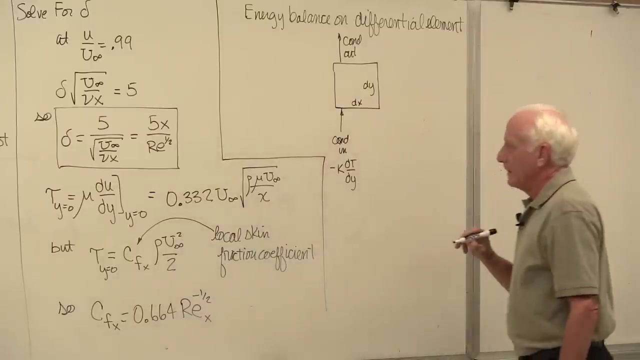 Okay. Okay, If it does, then there's going to be some conduction. Okay, so our conduction minus k, do it on a heat flux basis, minus k, partial t with respect to y. Then we'll have conduction out which is this plus the partial with respect to y, minus k, dT, dy times, delta times, dy. 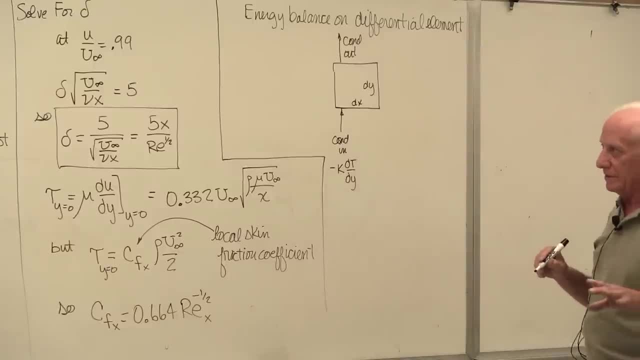 We're not going to worry about conduction in the x direction because if you're going to look at the diagram, there's a little temperature difference between the x and the y direction. You can use the dT dy to express the temperature of the fluid in the y direction, but we're 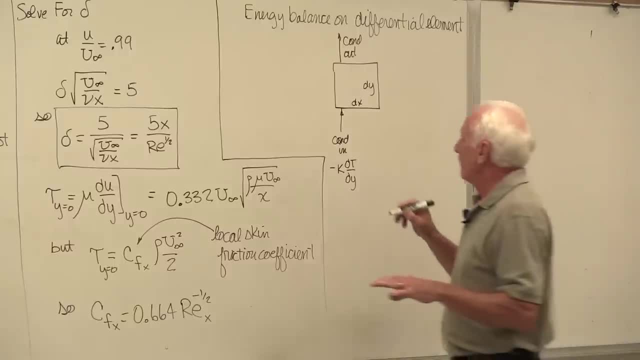 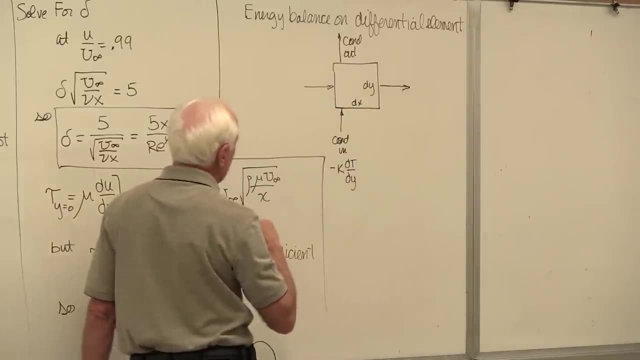 not going to be going through that Again, because temperatures are not a strong function of x as they are compared to y. But we do have some energy being brought in by incoming fluid and our little differential control volume. That energy is m dot, c, sub p, t, mE301.. M dot is rho av. Velocity is u. and velocity u. So we're looking at our solution here Now. we're looking at our solution. We're looking at our solution here. What we need to do is: we want to use our solution here. We want to be claimant about our solution. we want to be claimant about our solution. 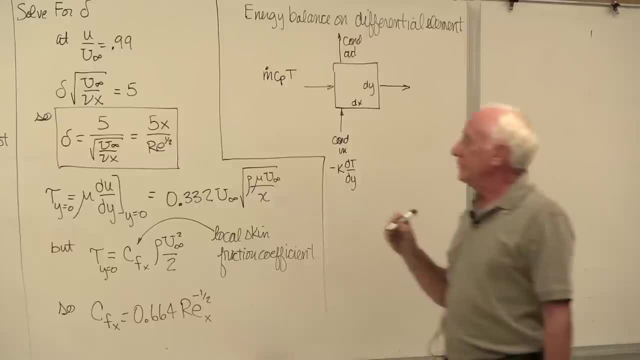 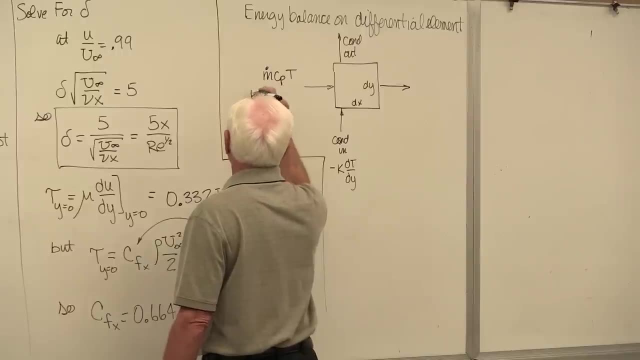 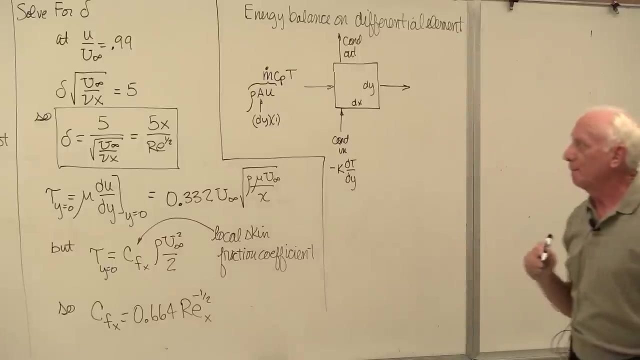 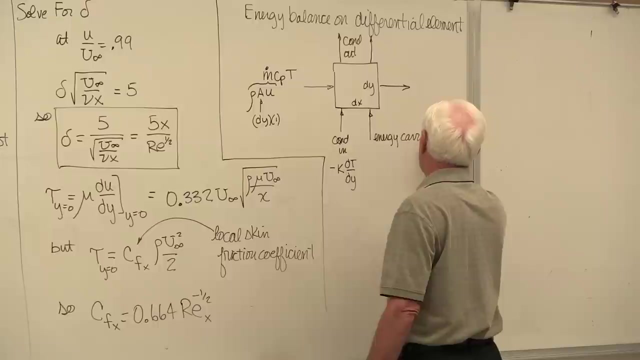 M, dot is row, AV, Velocity is U. The area is the vertical DY times 1.. And then you have energy going out In the Y direction. same thing In and out. Energy in And energy taken out as a function of the mass flow rate. Well, you put all those terms in the energy balance. 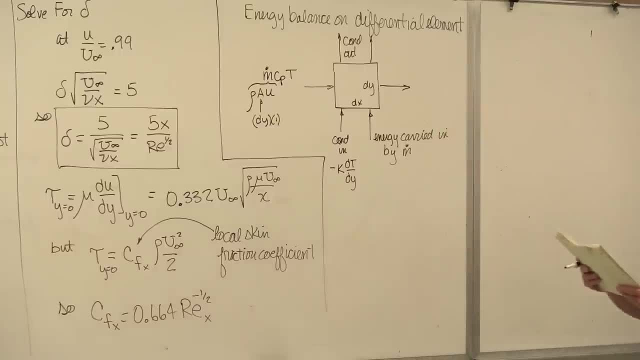 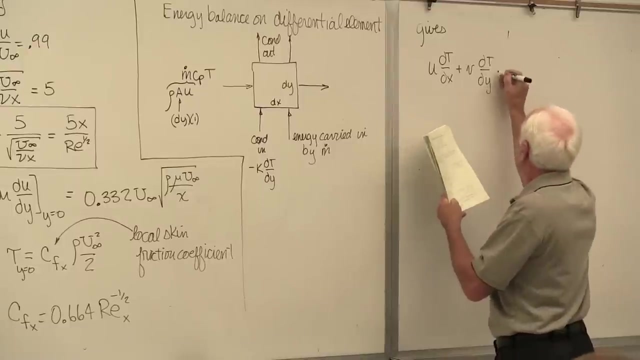 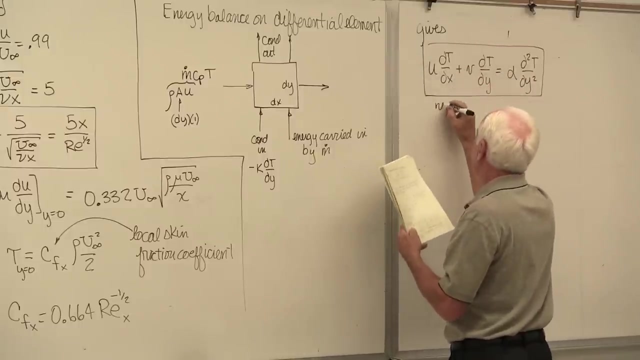 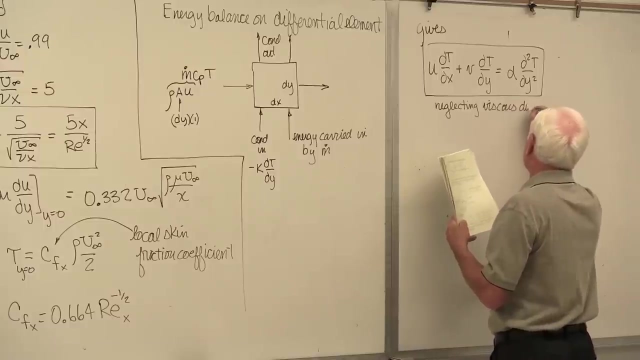 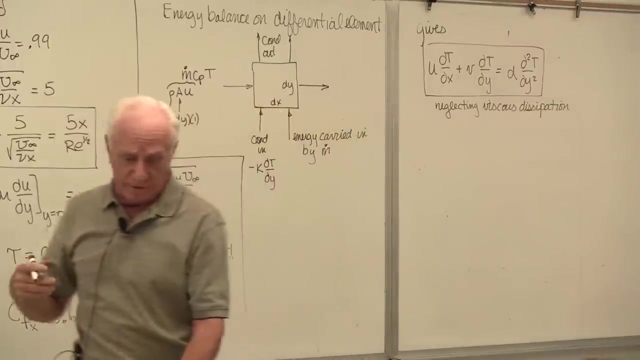 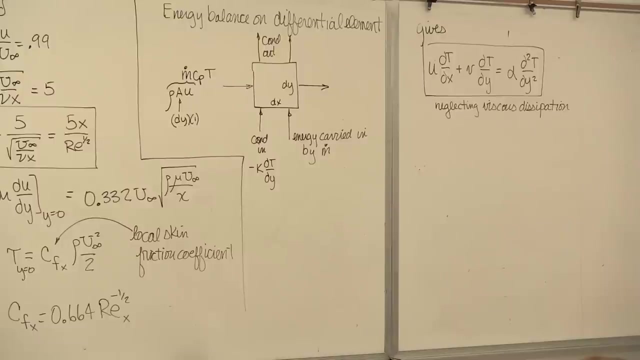 and we won't go through all the gory details. Our textbook does a good job of that And this gives this as your final result. And in that there's also sometimes there can be energy generated by viscous effects. You know, heating Space shuttle comes in from outer space previously, or any kind of. 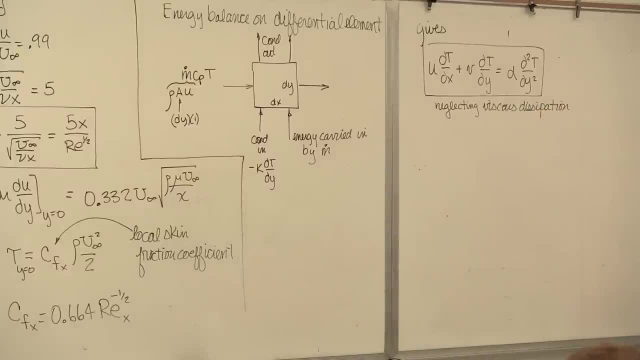 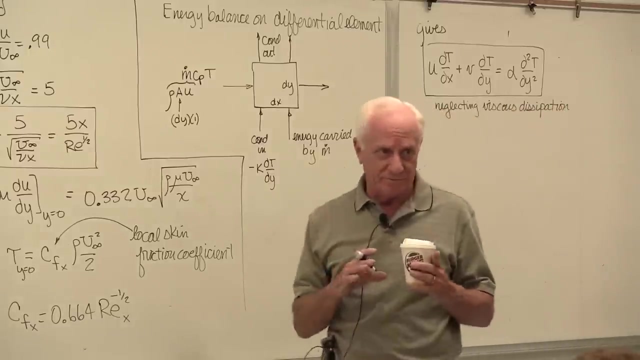 manned spacecraft And you see this glowing light. Yeah, there's a lot of heat being generated at the nose area of that particular vessel, But that's high-speed flow. We're not going to worry about high-speed flow here. This is not Mach number 5, okay, This is fairly low-speed flow, So we're not. 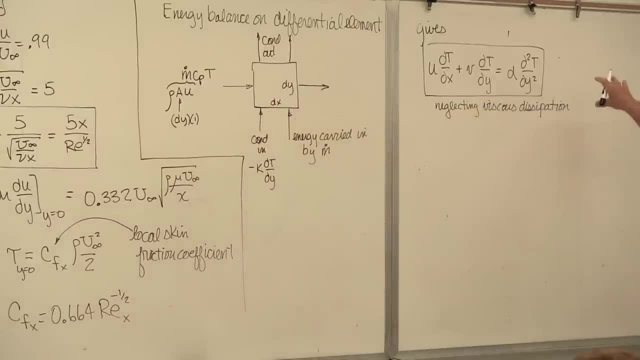 going to worry about viscous dissipation. That term disappeared. It's a mu term. It has mu in it, Okay, Okay, what's the object now? again, The object is to solve for temperature in the boundary layer as a function of X and Y. Where are these three equations valid? 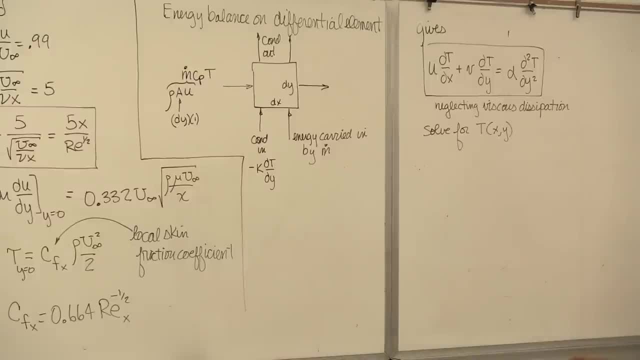 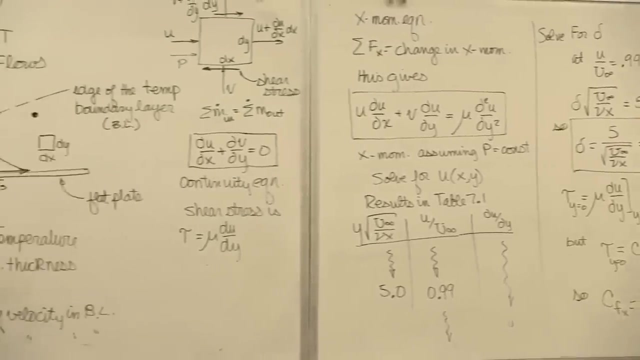 In the boundary layer either velocity or temperature. So if I put a big black dot in there and I say, okay, I want you to tell me the temperature in the boundary layer where X equals 5 centimeters, Y equal a half a centimeter, You could do it. then How Solve this guy? 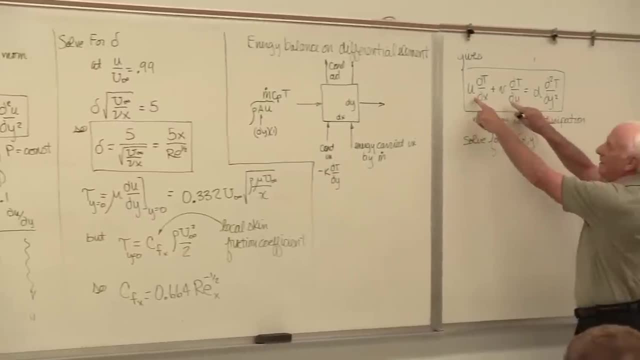 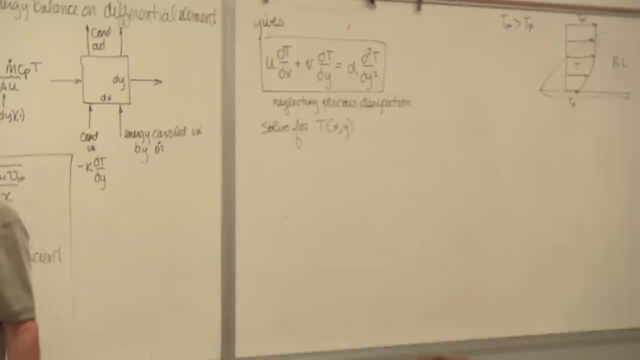 But to solve this guy, What do you need? I need to know U and V as a function of X and Y. Okay, there they are, at least U. And how did you get that? I solved momentum and continuity, So I take the that's. 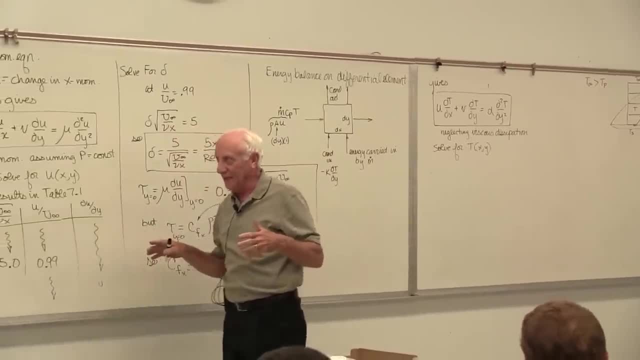 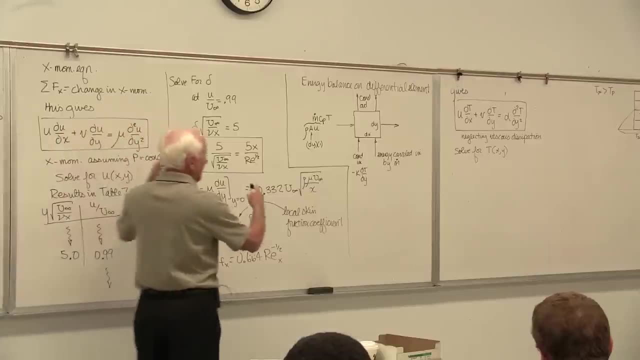 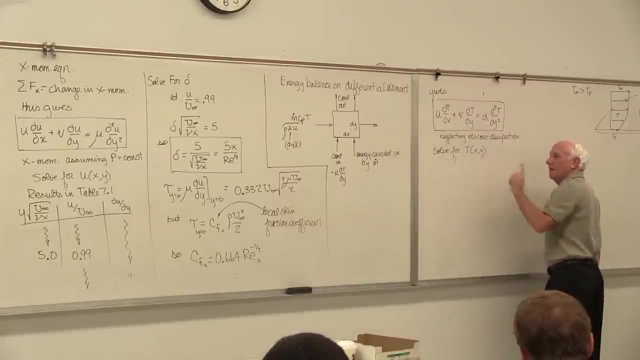 why the prerequisite on ME415 of fluid mechanics? Because you take the results of fluid mechanics from this and you put that up here from the temperature Temperature boundary layer and now you solve for T as a function of X and Y. Look how similar. 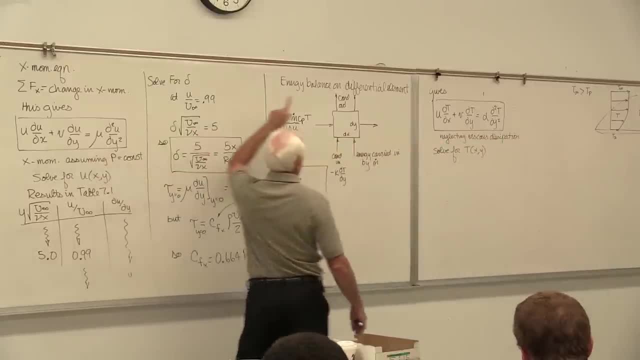 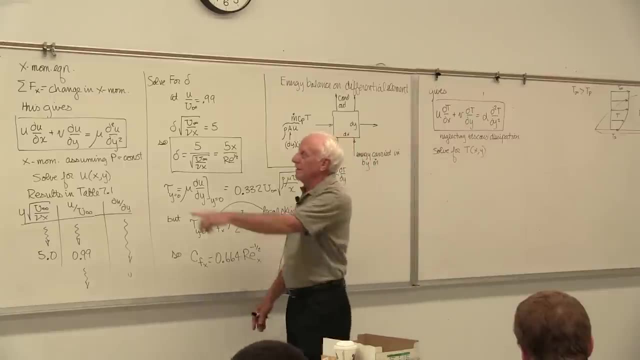 those equations are: U DU DX, U, DT DX, V DU DY, V DT, DY, A constant times D squared. U DY squared, A constant times DT squared, DY squared. Wow, They almost look like you. 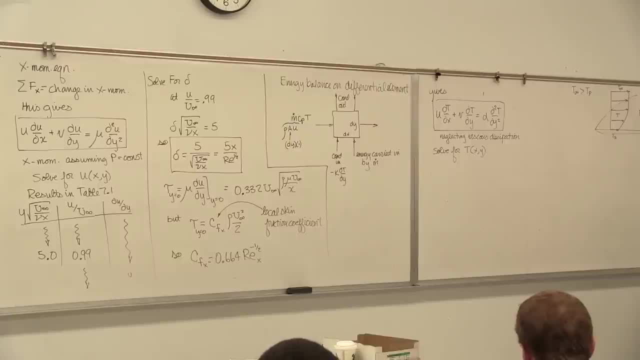 could solve one and get the answer for the other one because they're so similar. This is thermal diffusivity. This is wrong. This is kinematic viscosity. Okay, Yeah, Which means you know, there must be something important about that alpha and that nu. There must be. 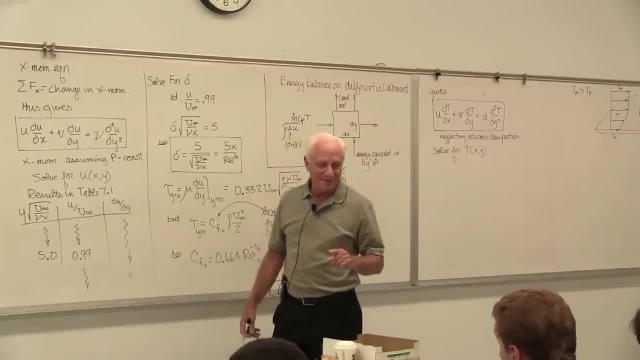 something important about that that connects those two. One solution might be connected to the other solution. Oh, and it sounds to me like this". 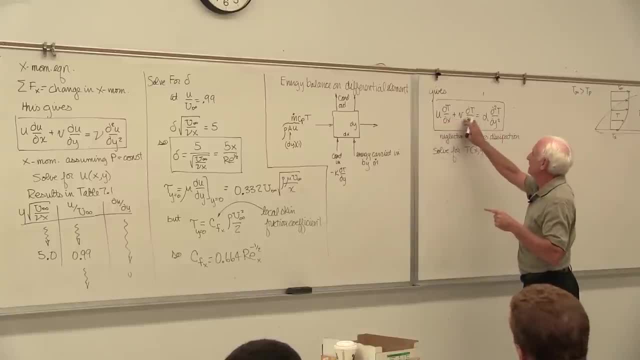 The only difference. they both have a U times this and a V times that, and this is an alpha and that's a nu. Yeah, that's right. We'll find out later on. There is a strong connection between them, Yeah. 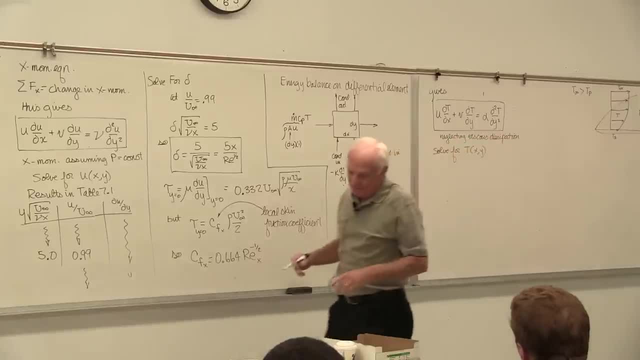 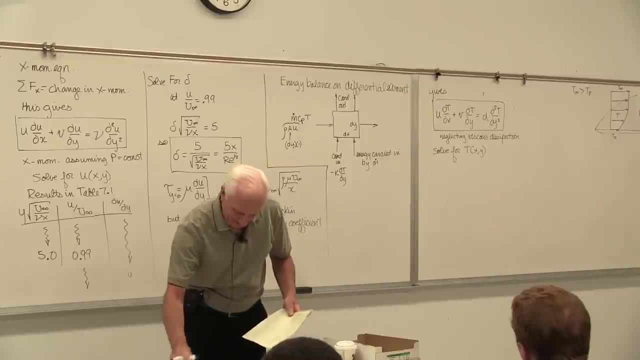 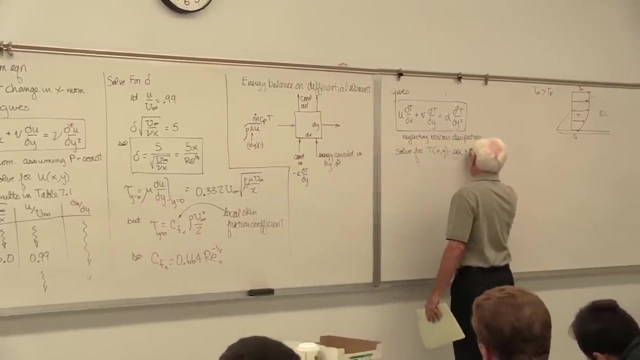 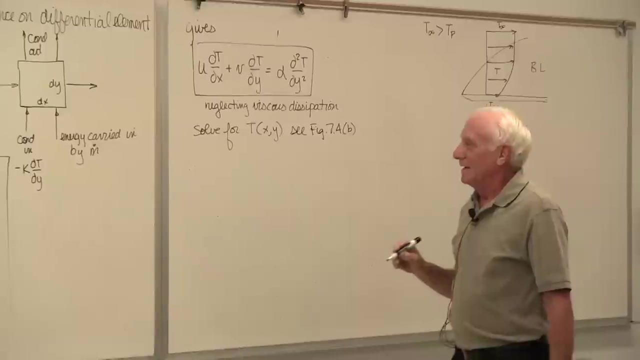 Okay, back to here. How do we find those temperatures? Well, not as neat and clean as we did for the velocity. They're given in figure 7-4b. 7-4b, It's a graph. it's a graph, okay. 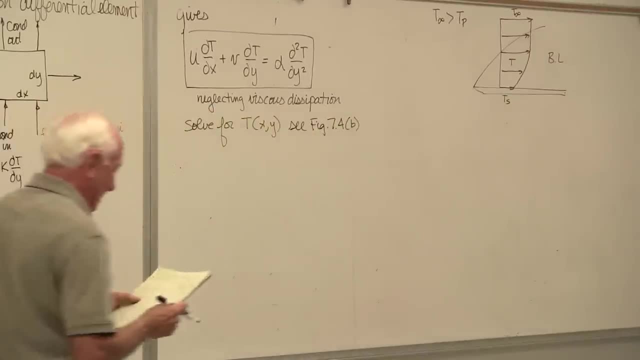 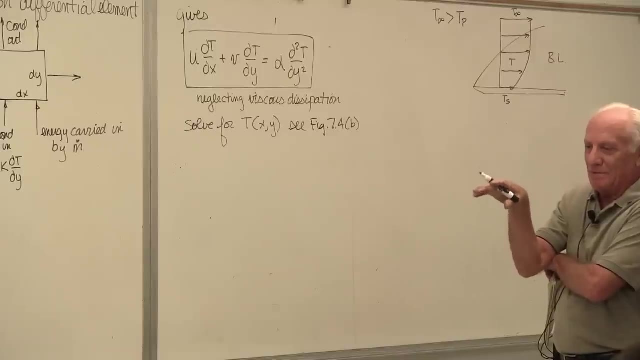 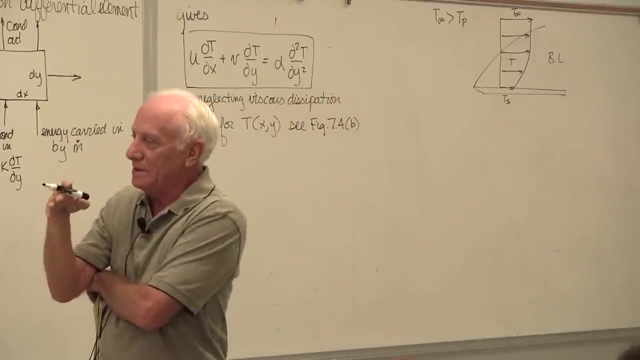 Okay, so now we have the solution for that Part of heat transfer. there's two main parts. part of it is to predict the temperatures in some particular situation. In a situation like this, we had it in conduction: Tell me the temperature halfway through a plate of thickness five centimeters and so. 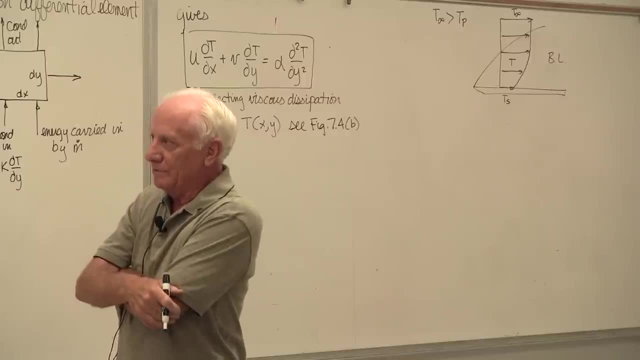 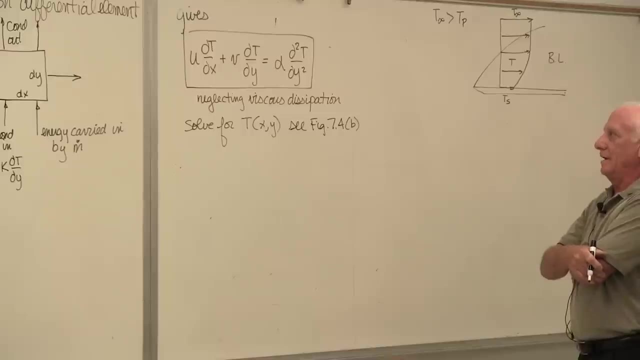 on and so forth. Find the temperatures somewhere. Number two, which is very important: find the heat transfer. That's why the course is titled heat transfer. Find the heat transfer. Okay, how do we find the heat transfer here? Well, all right, here's one way to do it. 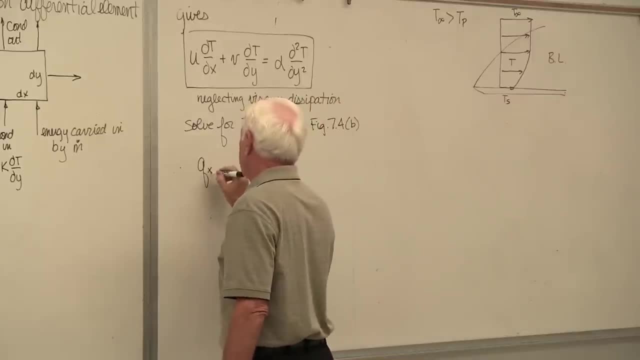 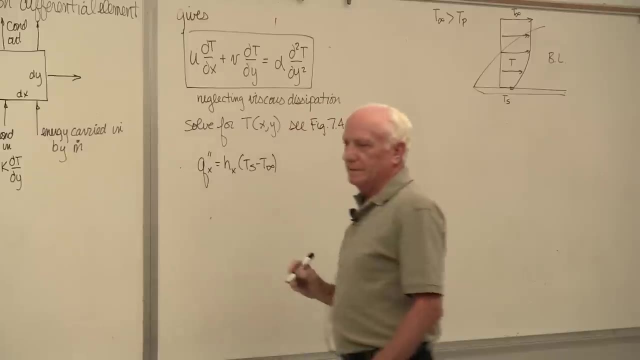 Q X double prime equal H X. Okay, Times T surface minus T infinity. T surface is constant, T infinity is constant. H is a convection coefficient. Chapter one, chapter one: Newton's law of cooling. Try and solve for H X there, okay. 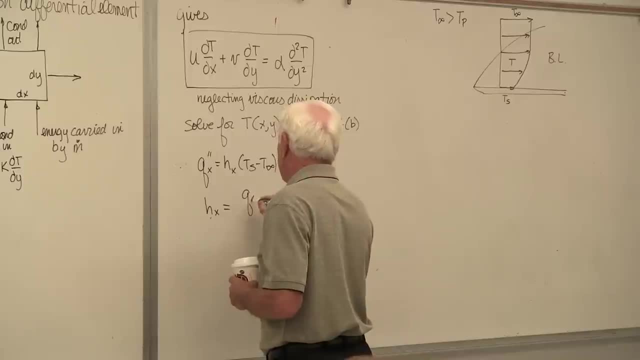 H X is equal to Q X double prime, T S minus T- infinity. Is that H X? No, because I don't know. Q X double prime. No, it's not. It's true, It's the truth, but it won't help me find H X. 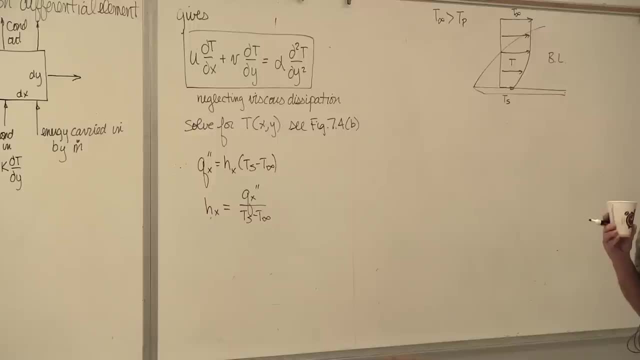 What does H X mean? by the way, It means the H value at a particular X location. It's called the local convection coefficient. The word local means as a function of X- Local convection coefficient. Okay, Local convection coefficient. 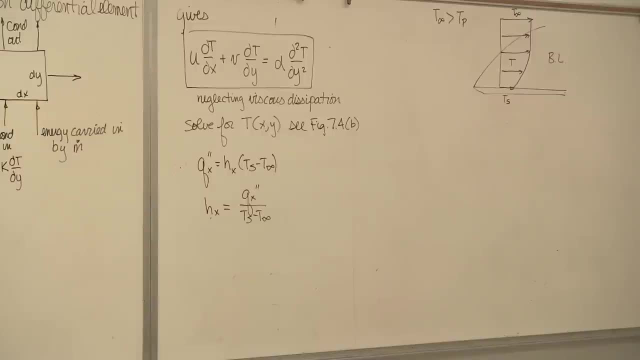 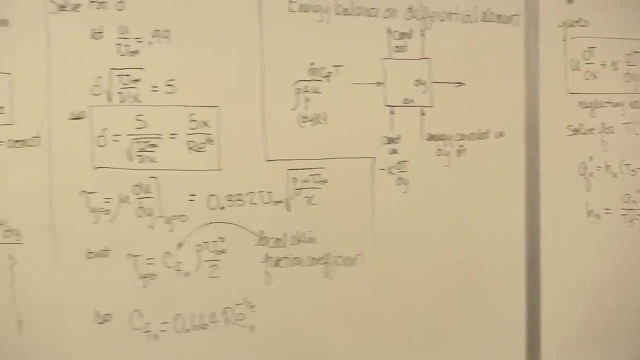 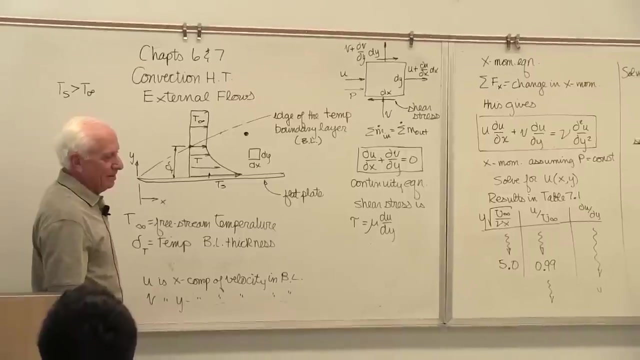 Well, look at the picture. Let's see now. How does the heat get out of that plate? The plate's hot, The fluid is colder. It leaves the plate right here where Y equals zero. And here comes the catcher. now You tell me the velocity of the fluid at the plate surface and I'll give you the answer. 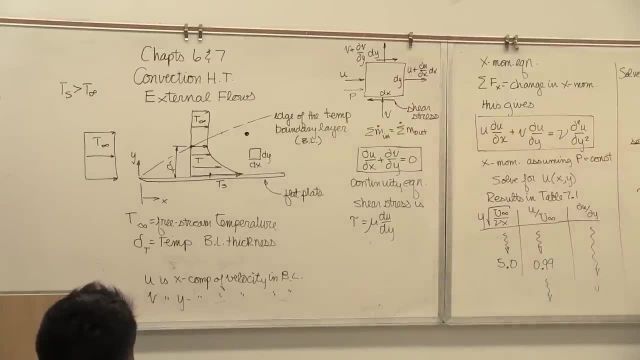 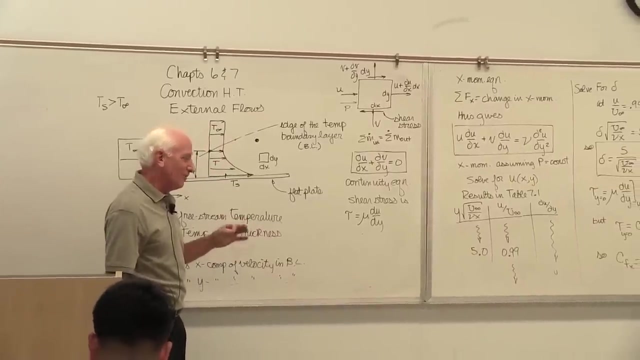 It's zero, The no-slip condition, The no-slip condition, ME 311.. That means the fluid is not flowing at Y equals zero. What does that mean? Oh, here it comes: Conduction. Conduction occurs where the velocity of the fluid is zero. 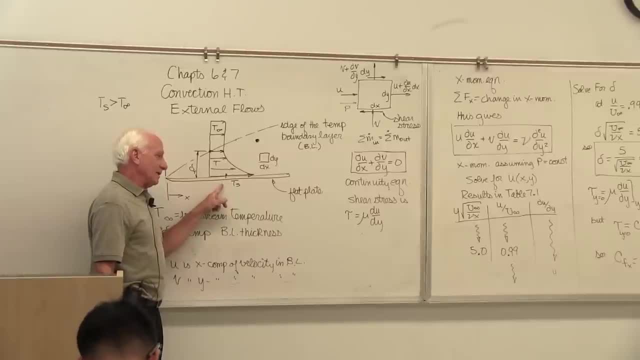 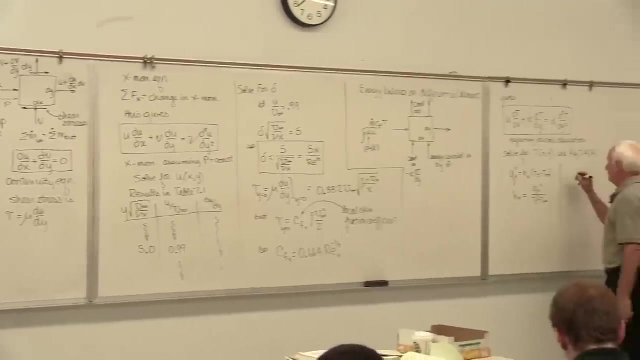 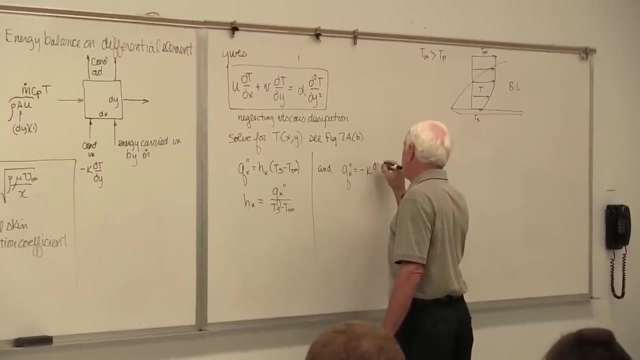 So the heat leaves the plate by conduction at Y equals zero and is carried away by convection to the fluid at T infinity. Here it is being carried away, the fluid to T infinity, But it leaves by conduction And QX double prime equal minus K, DT DY, where 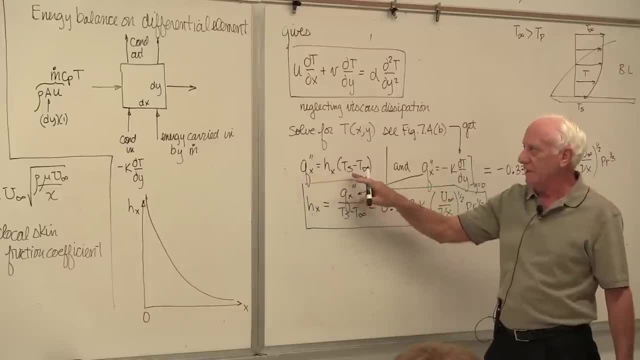 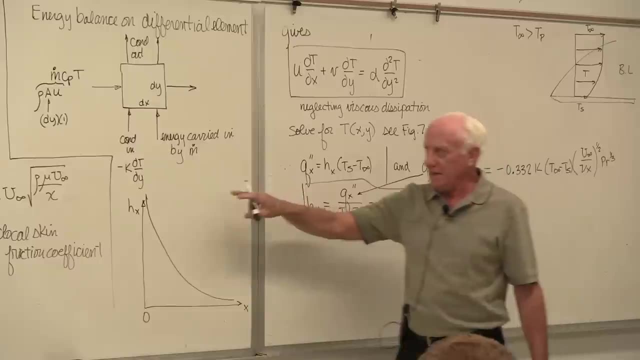 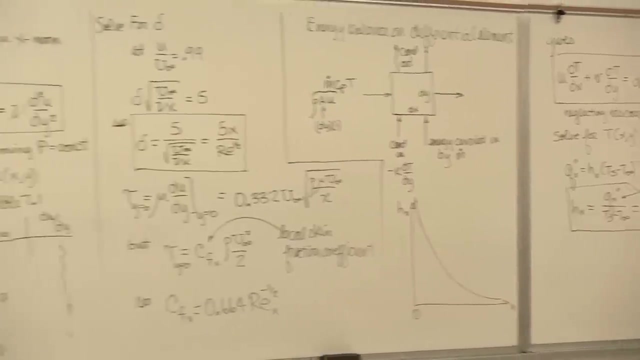 the greatest in flow over that flat plate. Well, don't forget: TS minus T, infinity is a constant. Q is the greatest where H is the greatest. So the answer is: the most heat transfer on a per square meter basis occurs at the leading edge of the plate. 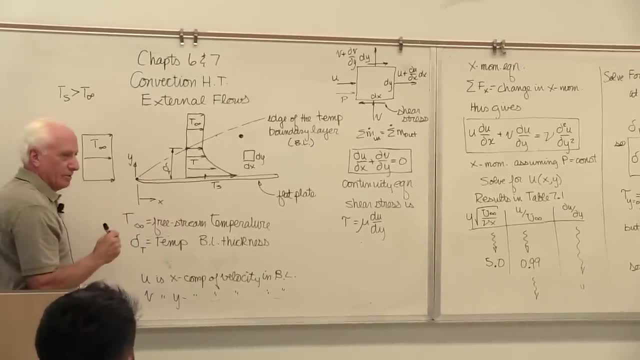 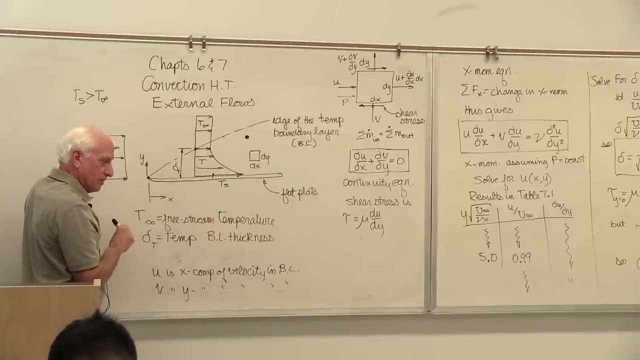 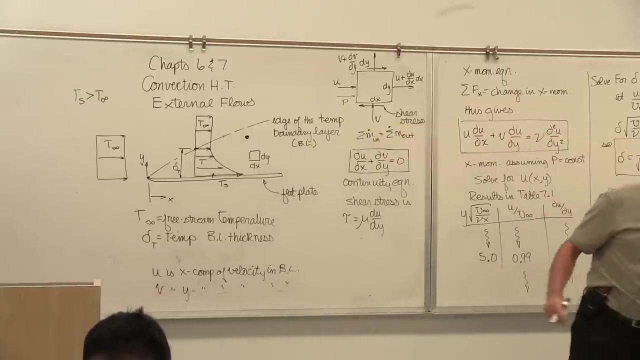 right there. That's where the biggest heat transfer occurs. As you go further down the plate, as X increases, the heat transfer goes down, gets smaller and smaller and smaller. Some people say it's due to the thickness of the boundary layer. getting bigger It's. 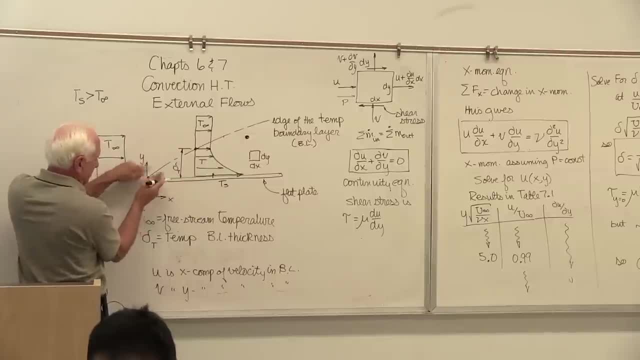 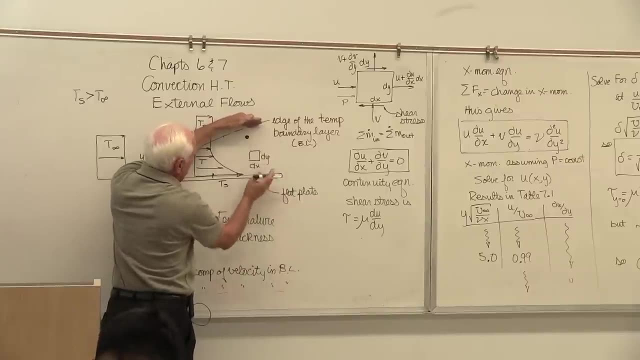 an insulating effect. So here's the boundary layer. The thickness here is zero. It gets bigger and bigger and bigger. The thicker the boundary layer gets. by that they mean the Y dimension, delta. the thicker it gets, the less heat is being transferred from the 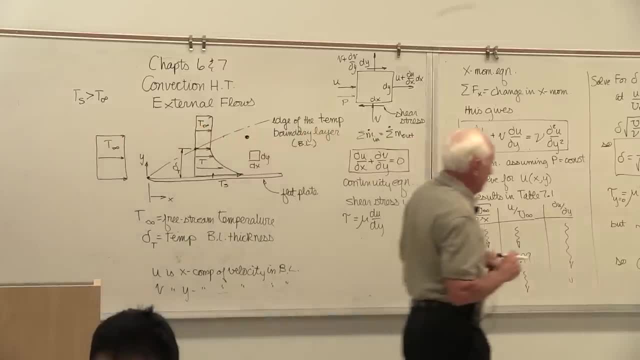 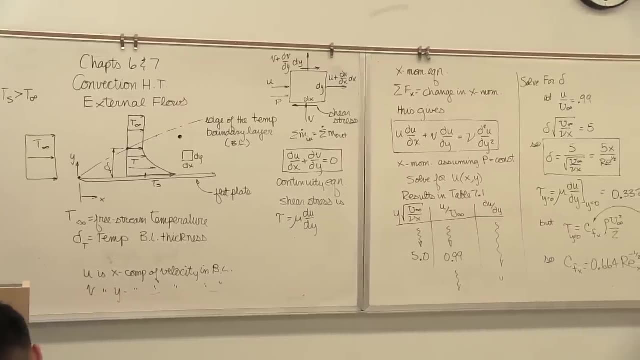 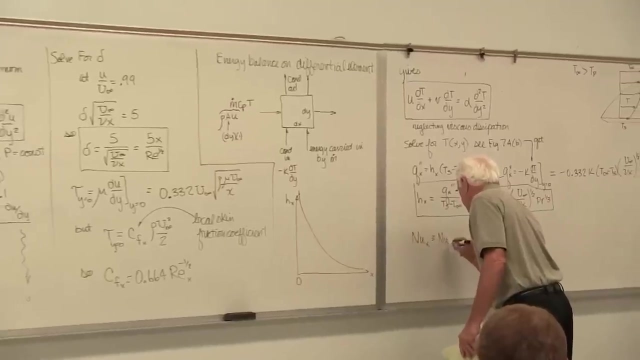 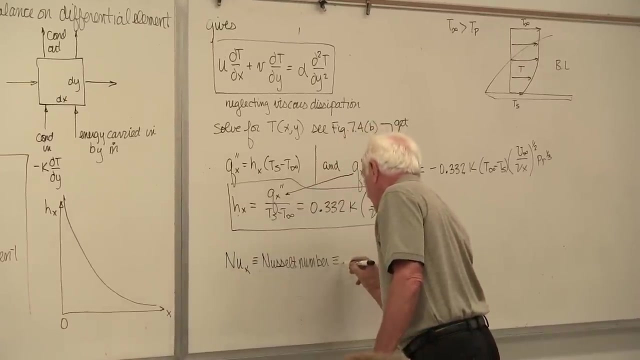 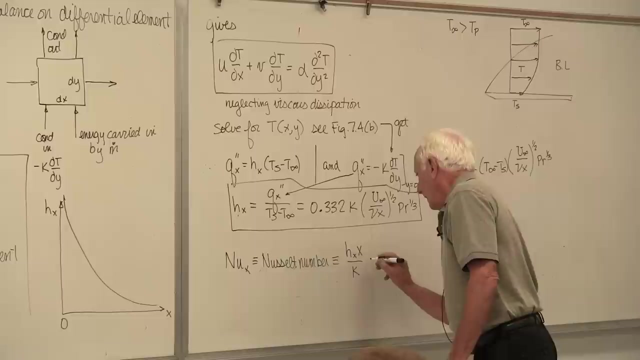 plate. Okay, All right, So that gives us H. Next We bring in a new dimensionless variable called the Nusselt number. Dimensionless, Okay. It's defined as H X multiplied by X over K, And if you put that H sub X from here down, 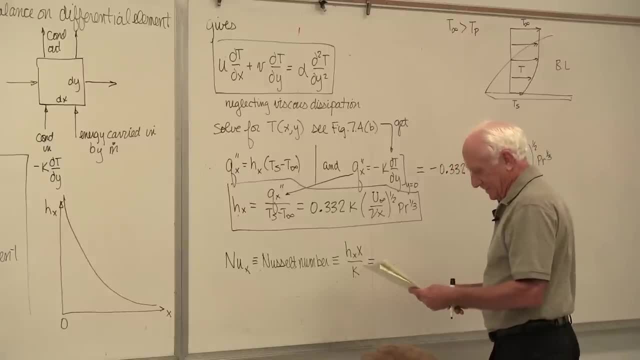 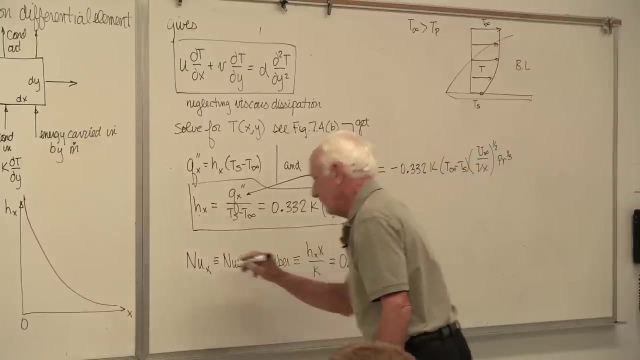 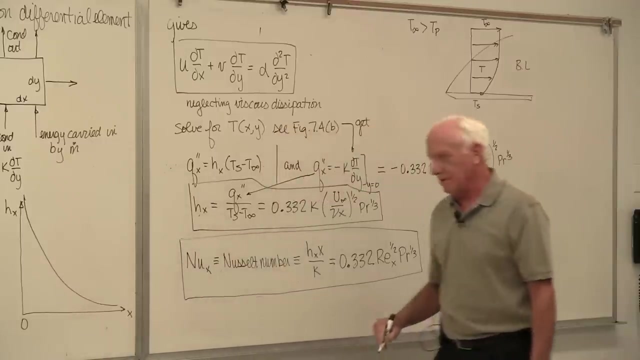 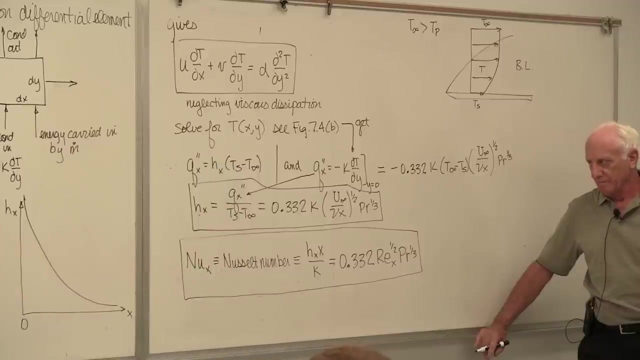 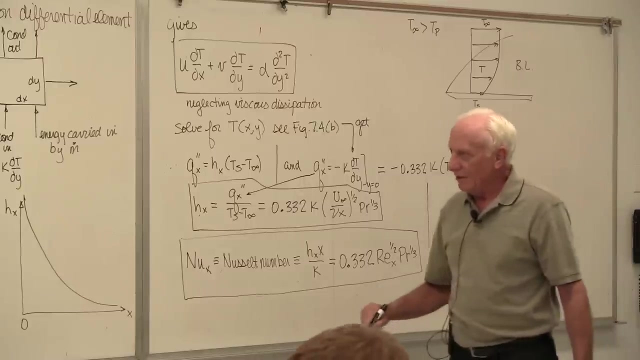 into here, you end up with this equation: Okay, So this is the dimensionless form of the convection equation. Three dimensionless parameters: Reynolds number, Prandtl number, Nusselt number, And the last thing we have is: what is delta for that picture over there? delta T. 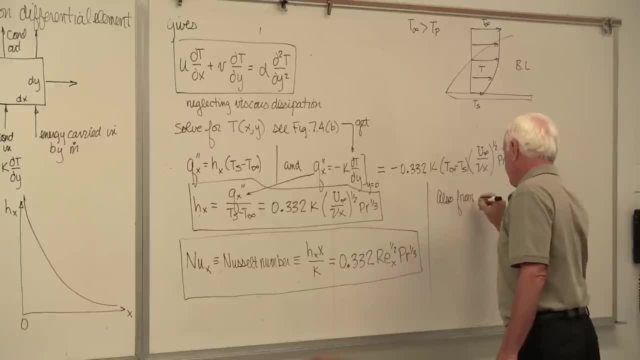 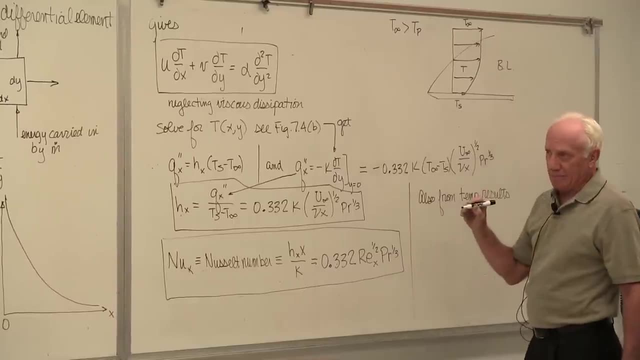 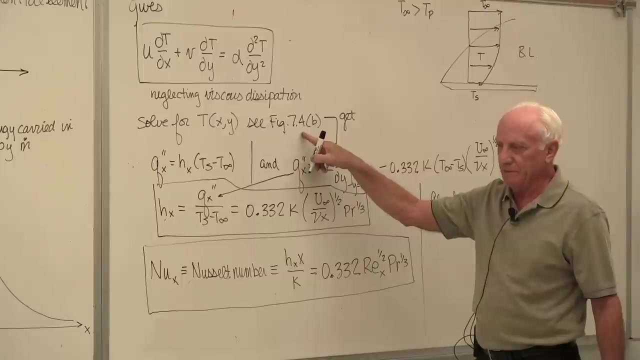 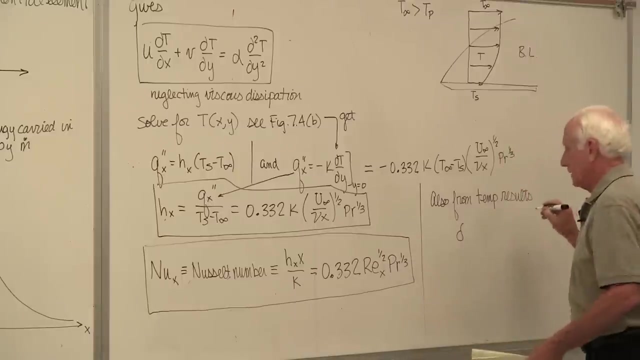 Again the 99% rule. go to the graph, see where the temperature approaches 99% of the free stream temperature and that gives you delta T. 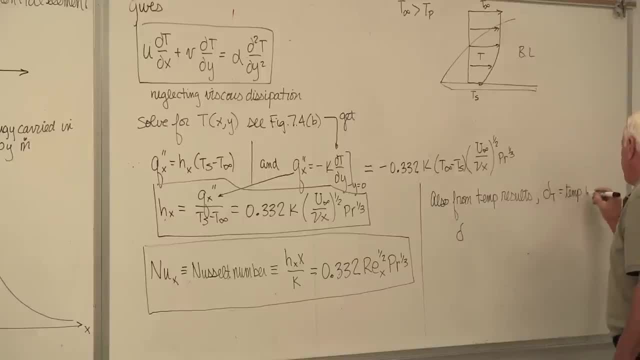 So delta over delta T is about equal to Prandtl to the one-third. So the first step is: you find delta, delta right there, Step one. let's go to step one. 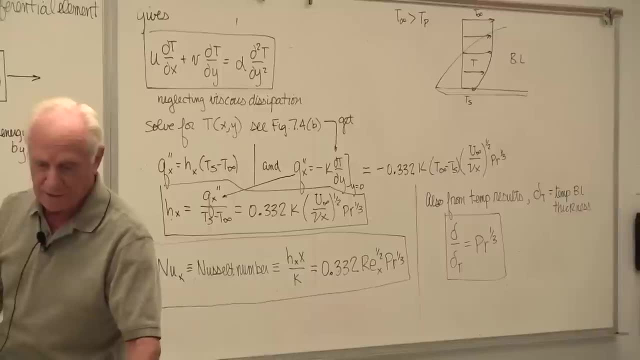 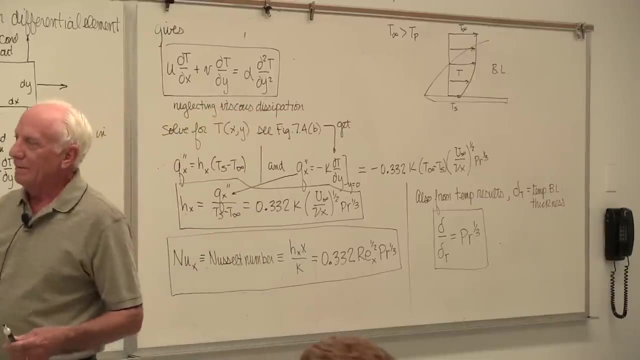 Step one of these problems: calculate the Reynolds number. don't forget fluid mechanics. Step one: always calculate the Reynolds number, tremendously important. okay, Get the Reynolds number, We're going to find out. now, don't forget all these boxed equations over here, except 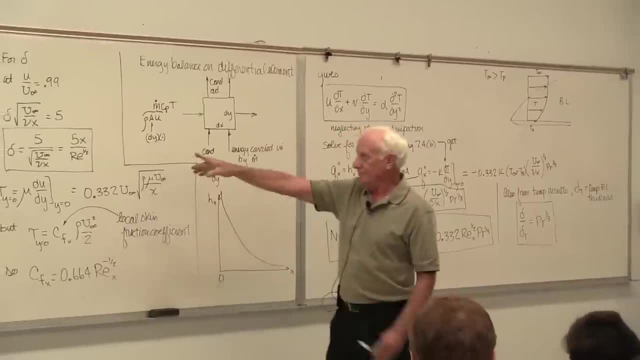 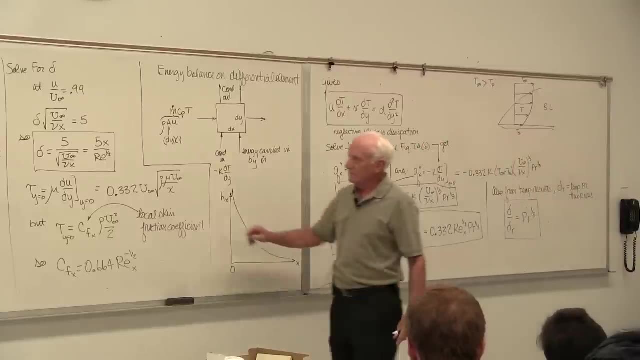 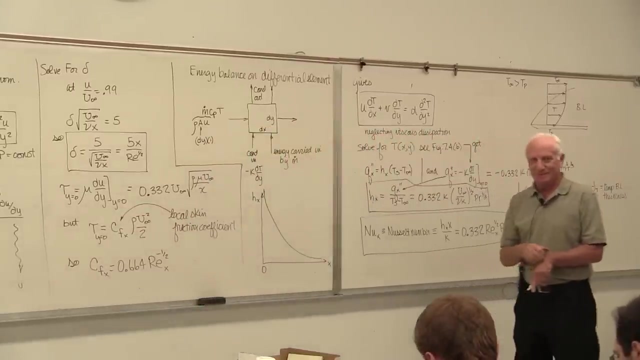 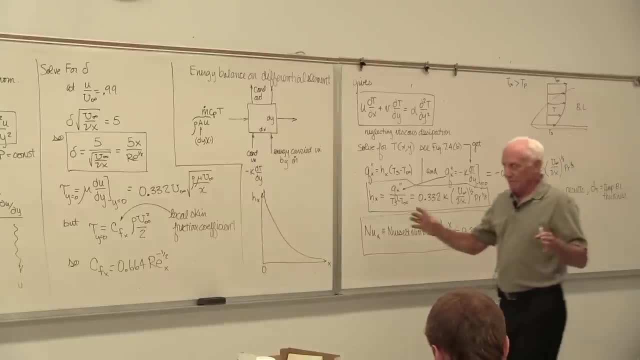 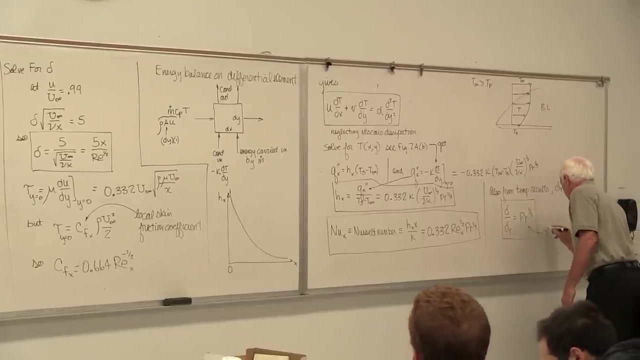 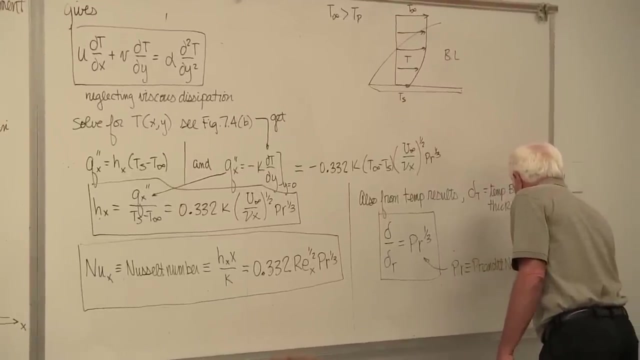 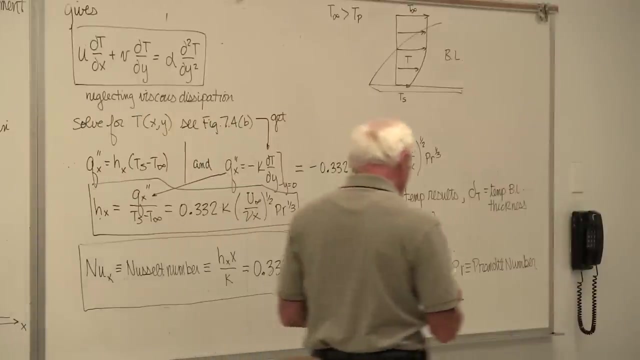 Get the Reynolds number. put it in here. add a particular x calculate delta. put that delta over here. put the Prandtl number in Prandtl number- Prandtl number and my Prandtl number. Two ways to write it. we'll do it this way first. 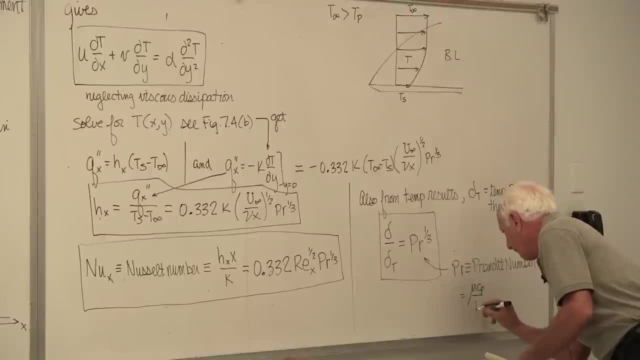 Our mu Cp over K, which is also equal to our nu over alpha. nu over alpha- Isn't that interesting? The ratio of nu over alpha is to find the Prandtl, Okay, Okay, The Prandtl number, and it appears right here. and remember that I said. 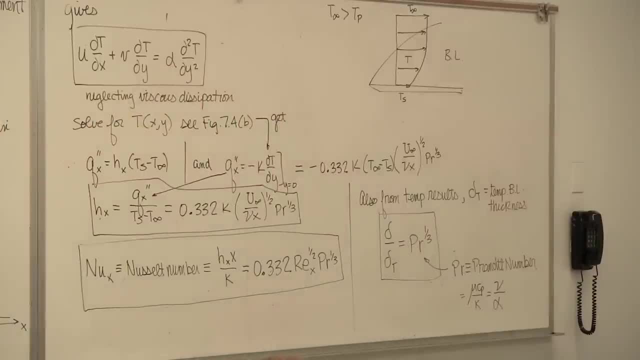 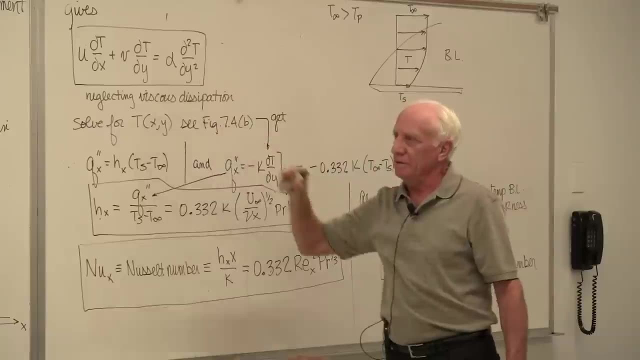 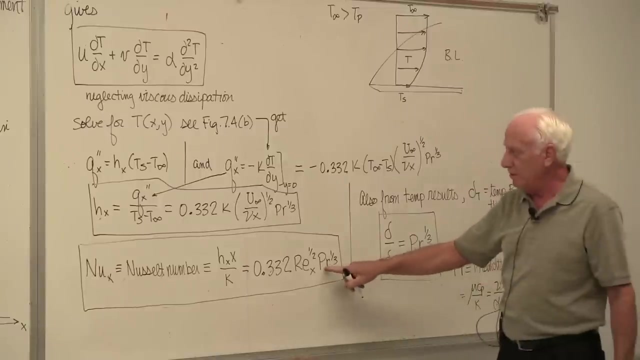 There's alpha and there's nu. There must be something about that, because both of the equations are very similar, except one has a fluid property, nu. the other one has a fluid property, alpha. yeah, It pops up here. We call it, we give it a special name, the Prandtl number, and it pops up in the equation. 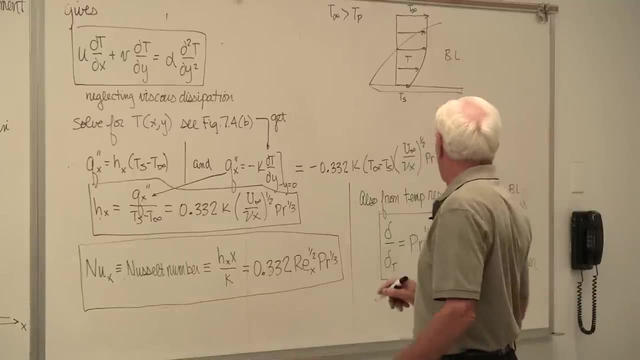 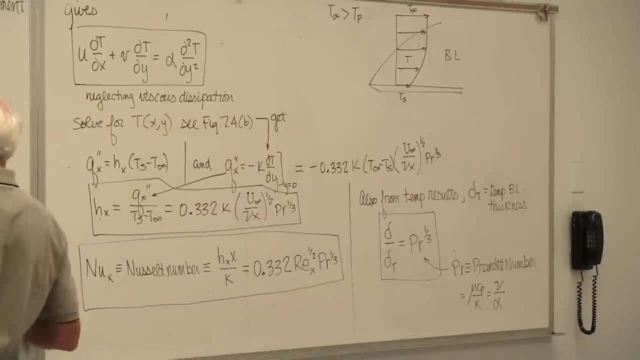 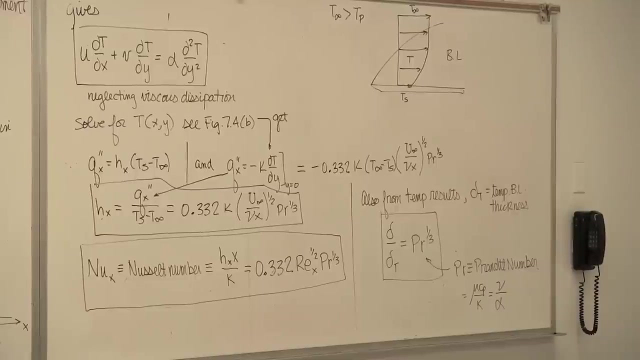 here. Okay, All right, We got that. We got that. Let's take a look at Prandtl. Okay, Let's take a look at what that means about the relative size of the boundary layers. I'll put that right here. 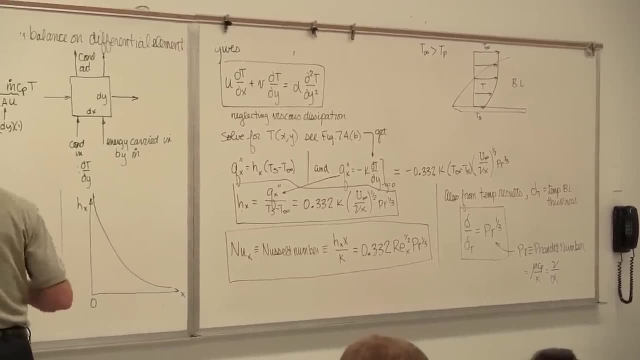 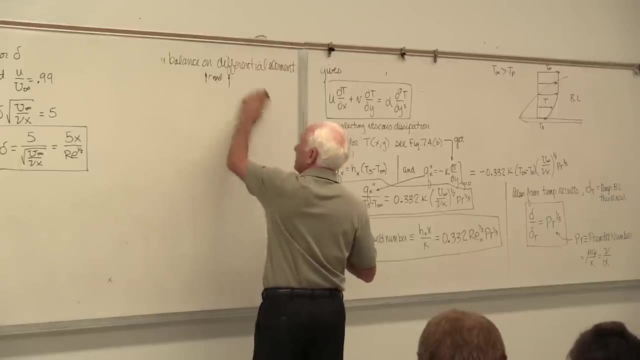 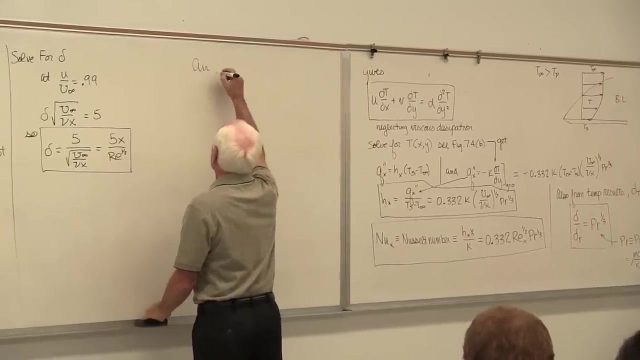 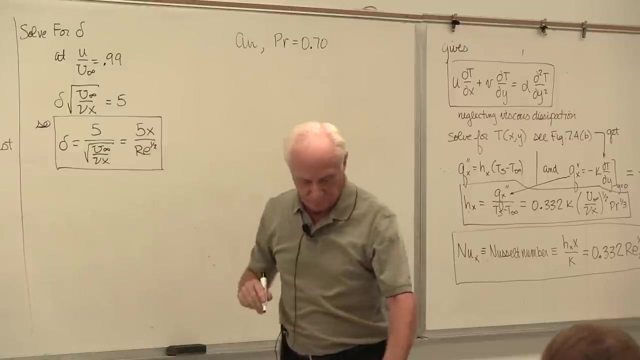 Okay, Let's take a couple of fluids at normal conditions, ambient conditions, temperature. Okay, Let's take air: Prandtl, Prandtl, Prandtl, Prandtl, Okay, Okay, And remember the Prandtl number is, at general conditions, about 0.70.. 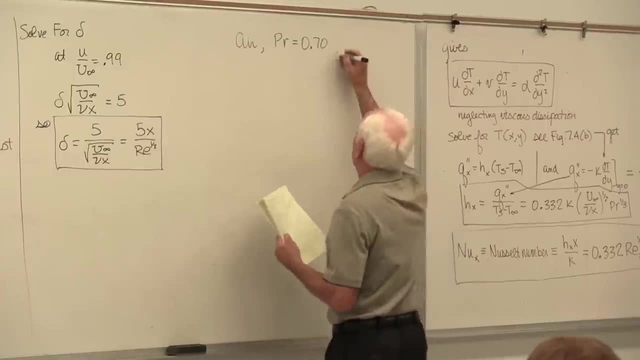 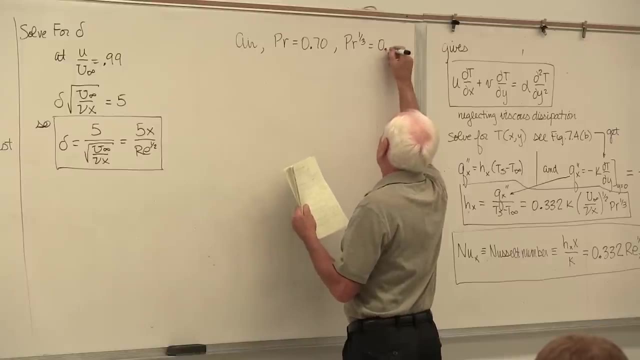 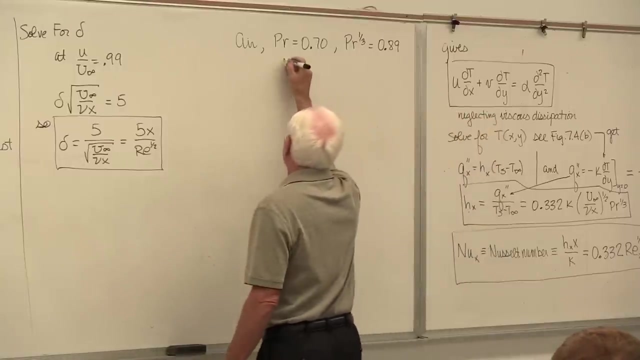 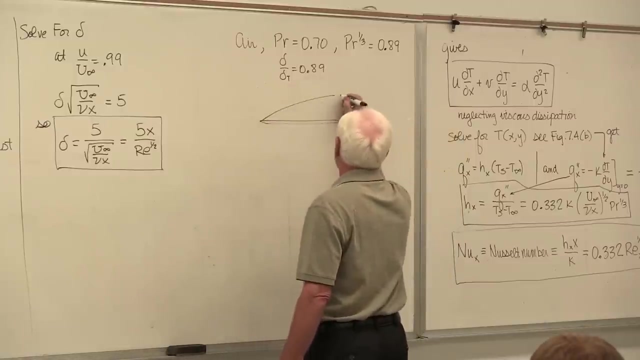 So let's look at what the Prandtl to the one-third is About: 0.89.. So that tells me that delta over delta T 0.89.. Okay, All right, Delta T is bigger. Here's the velocity boundary layer, and then our Delta T is bigger. Let's 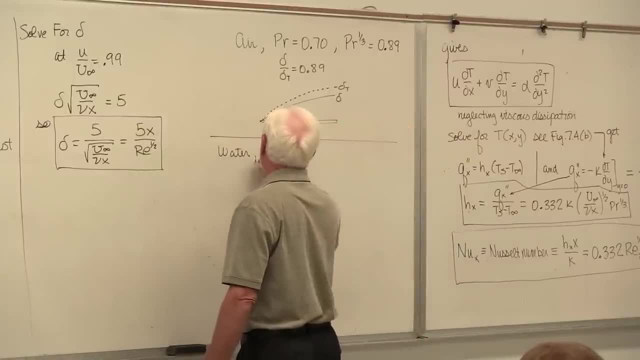 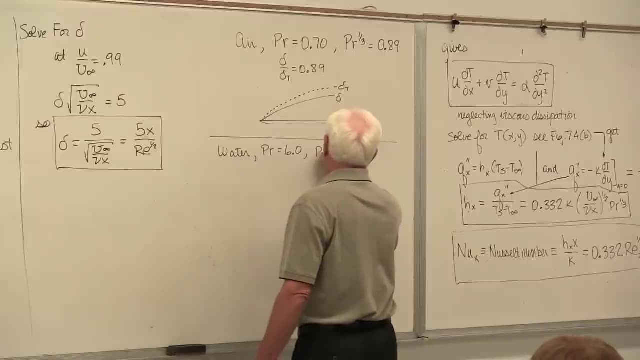 take another popular fluid water: Prandtl number at normal conditions around 6.0.. Prandtl to the one-third 1.8. That means Delta over Delta. T is 1.8.. So in that case let's show. 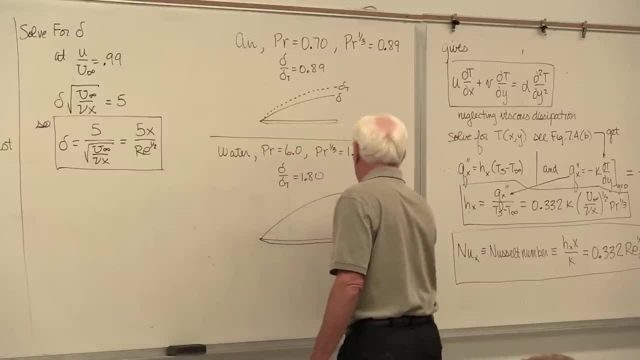 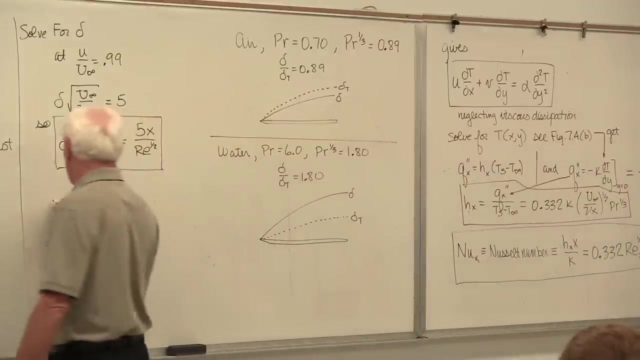 Delta Delta is up here, and the temperature boundary layer then would be Delta over 1.8.. So there's the relative sizes of the two boundary layers. Notice: Delta is about double Delta T. And now let's take another popular fluid: oil For oil, the Prandtl number is about 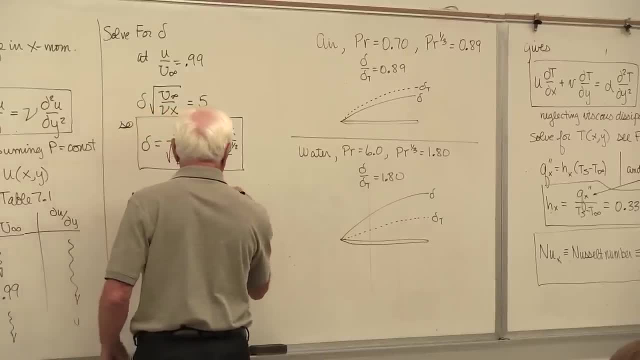 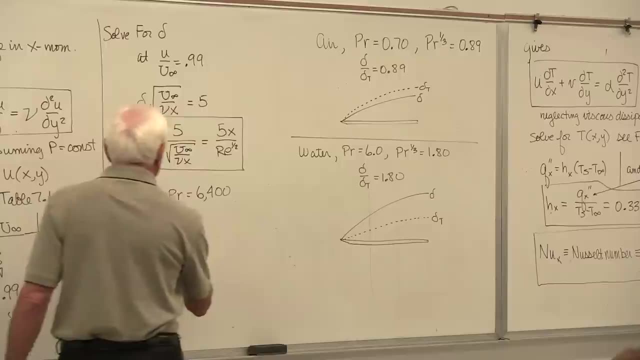 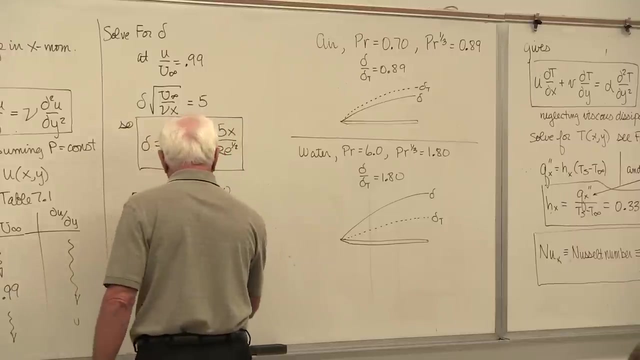 __. Alma is very, very large, 6,400.. Prandtl to the one-third, 18.. Delta over Delta, T is 18.. So here's the flat plate boundary layer, delta. Here's a temperature boundary layer. down here, Boy, the velocity. 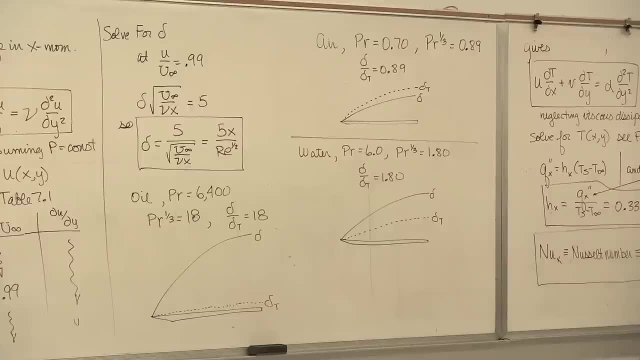 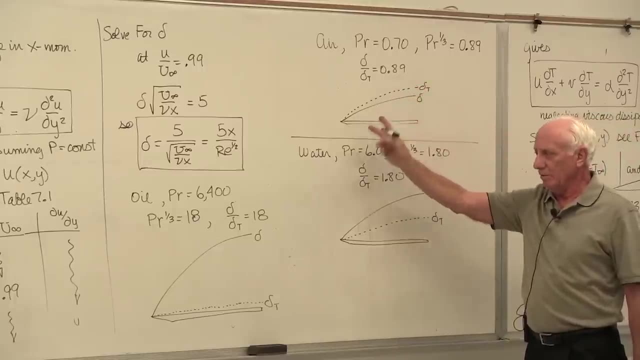 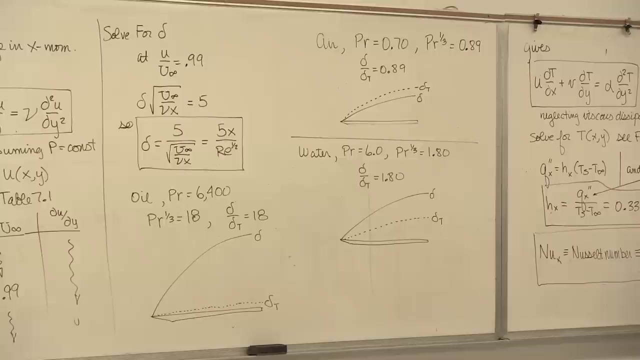 boundary layer is tremendously thicker than the temperature one. Of course. oil is very, very viscous. Air is not very viscous at all. No surprise: Oil, real viscous Water- two to one ratio at normal conditions, Okay. So that shows how those thicknesses here vary. 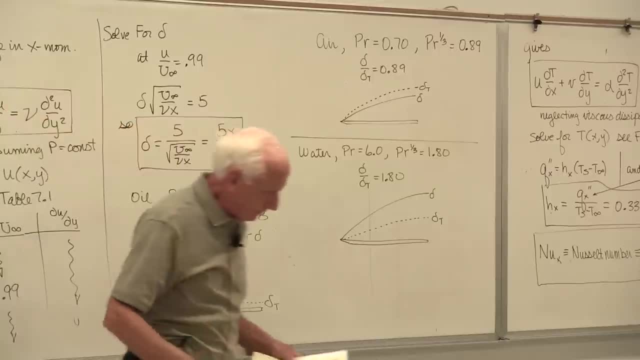 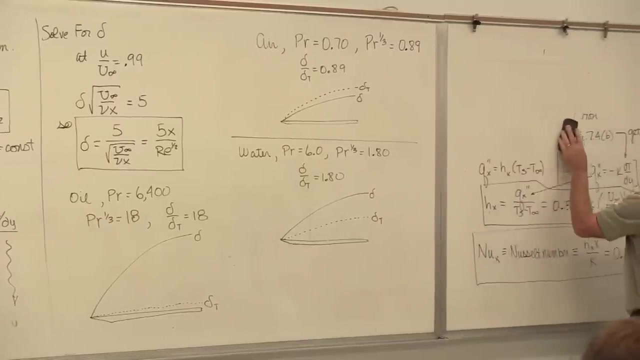 Delta, T and delta in the picture right there. Okay, Now one last thing. This is all for laminar flow. So these equations over here, laminar flow, don't use them in turbulent flow. Okay, Okay, Okay, Okay. 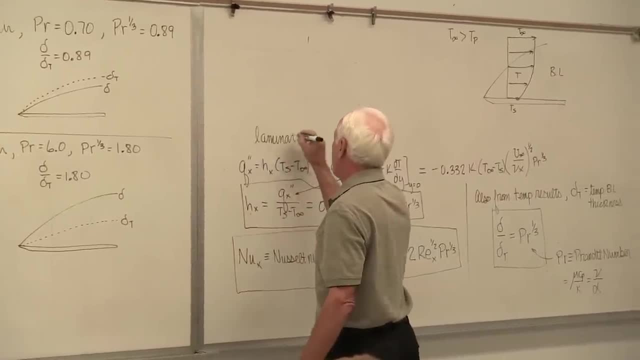 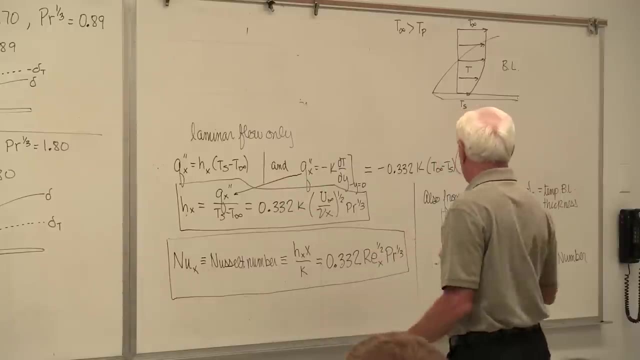 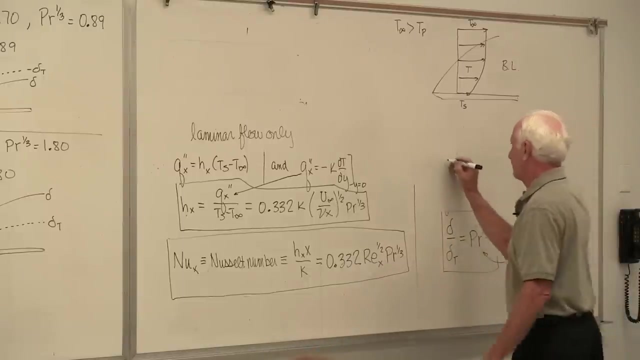 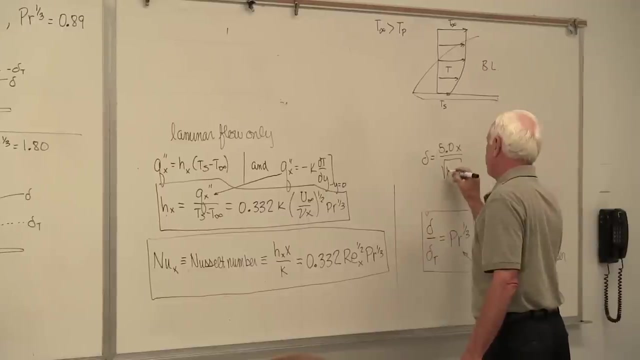 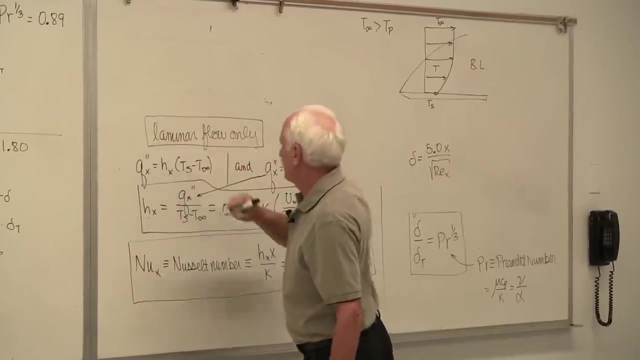 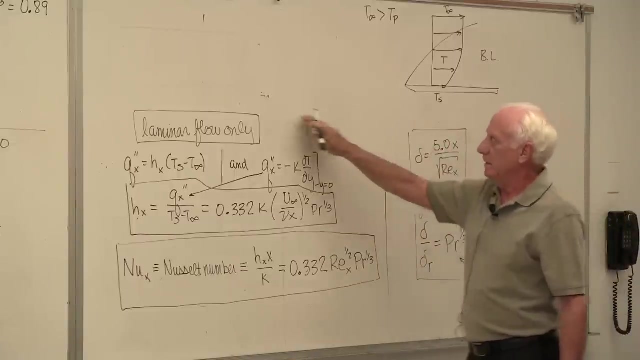 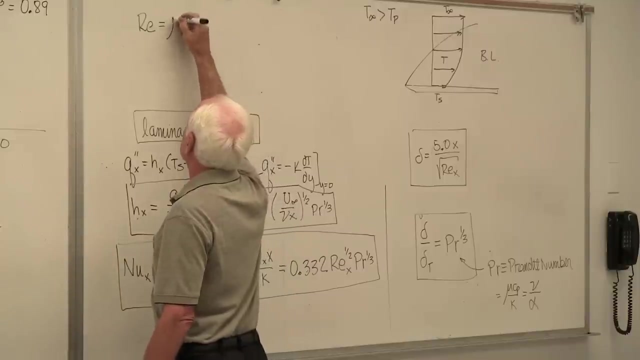 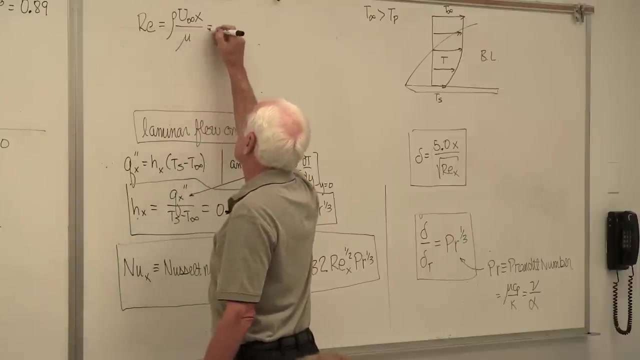 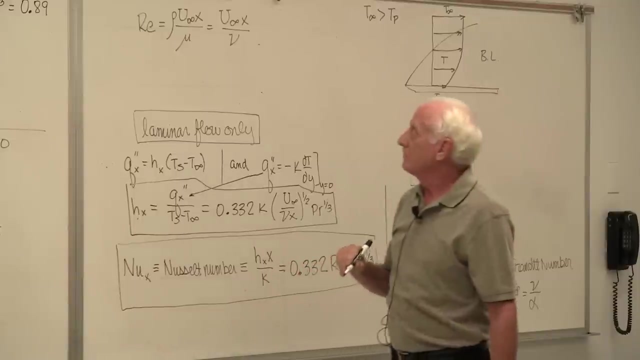 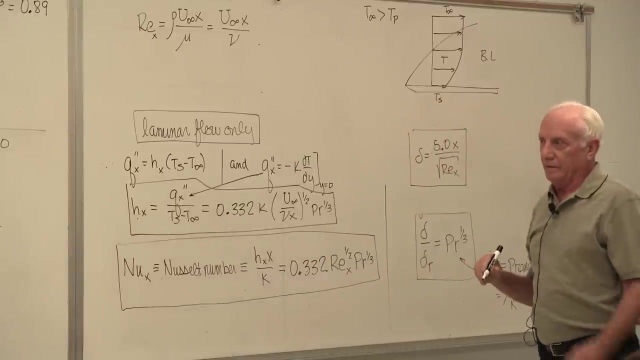